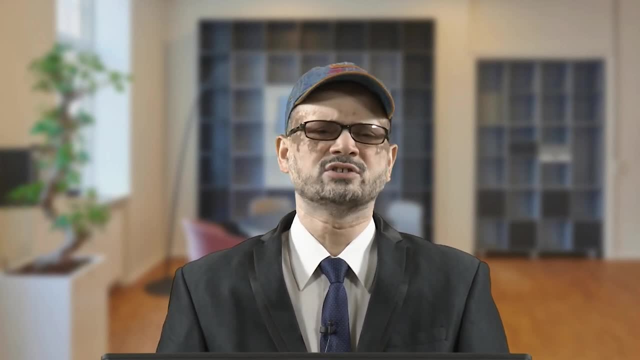 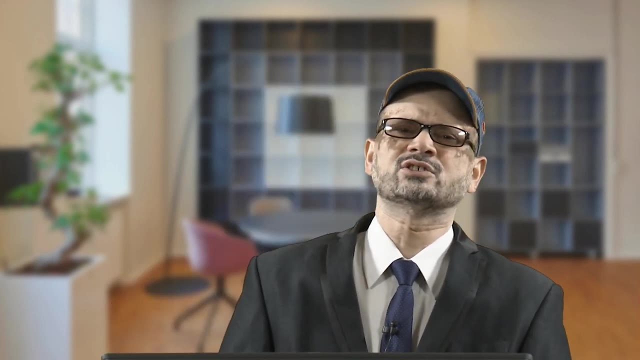 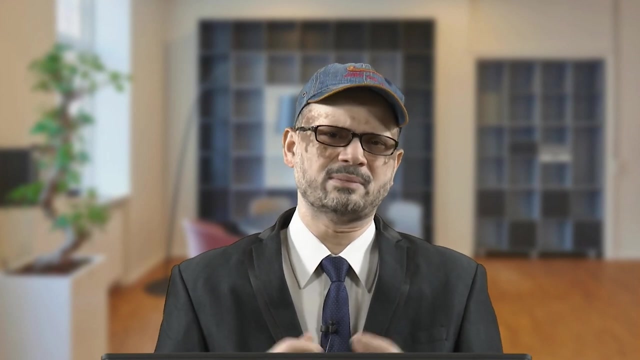 So there also there is a phenomena of phase change. So you will have, if you are trying to, you know, join two pieces, So initially they are in solid state, solid phase, Then once you heat them, I mean a certain zone is heated, then that, you know, converts. 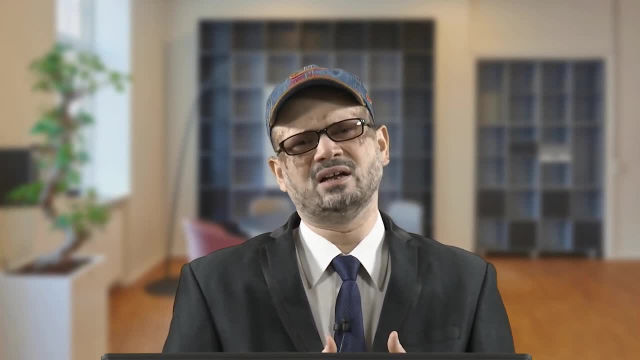 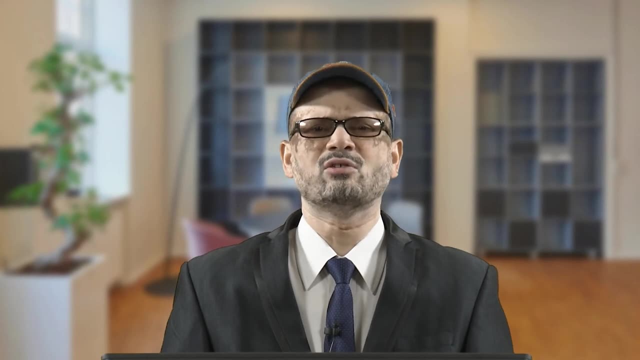 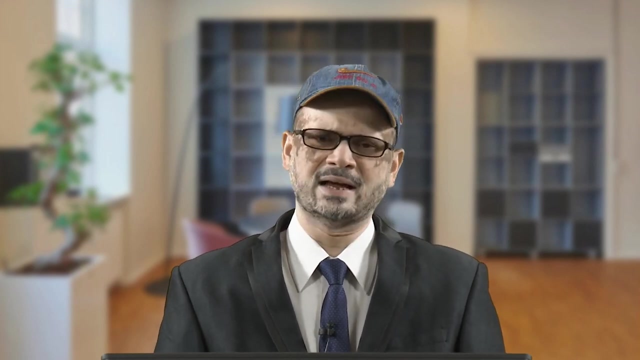 to liquid phase and further. as there is change in temperature, drop in temperature after being exposed to surroundings- Then there will be further transformation from that. Okay, So phase transformation from liquid phase to solid phase. Now we all know that this is all governed by certain principles. 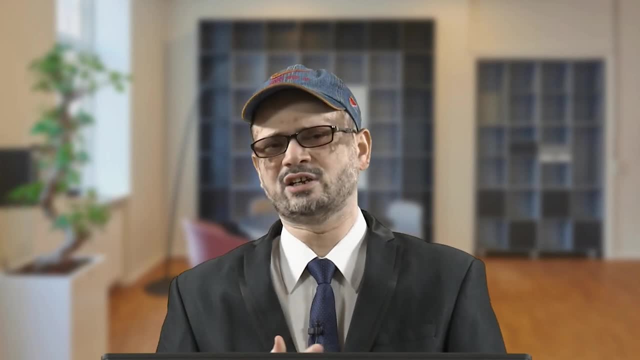 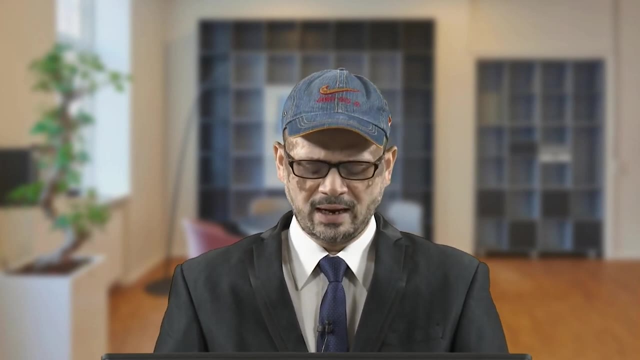 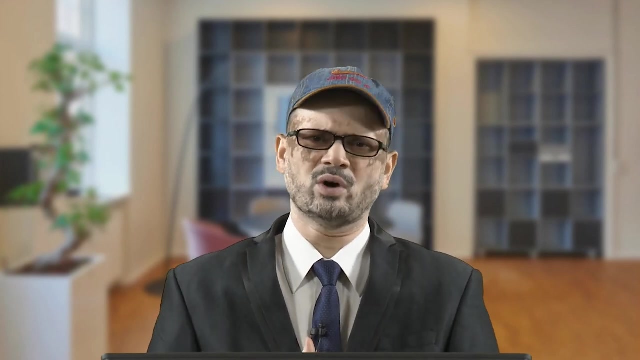 Why certain material is in solid state or in liquid state at any temperature. this is all governed by- you know the free energy concepts And how there will be phase transformation. what will be the mechanism of phase transformation? with what you know, way Okay. 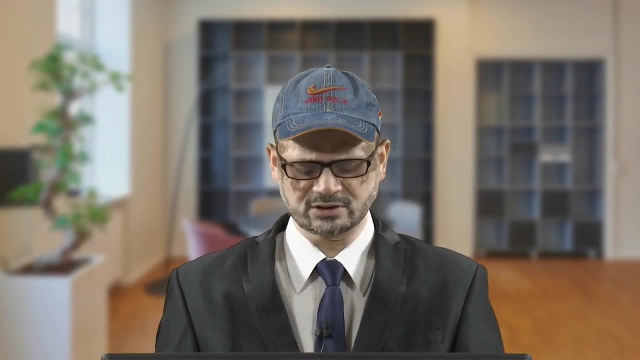 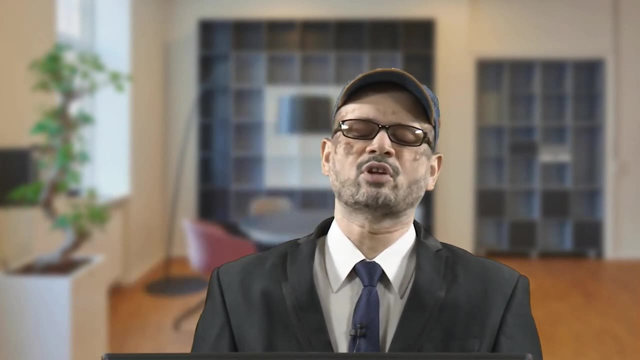 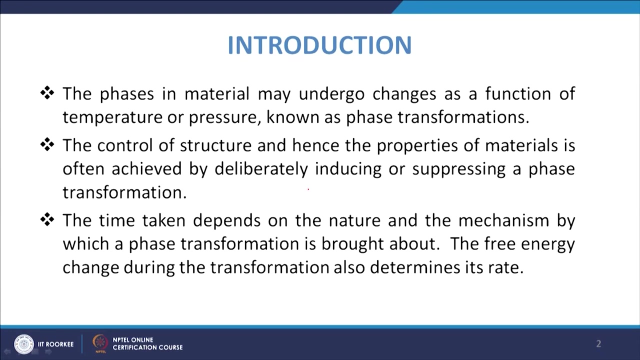 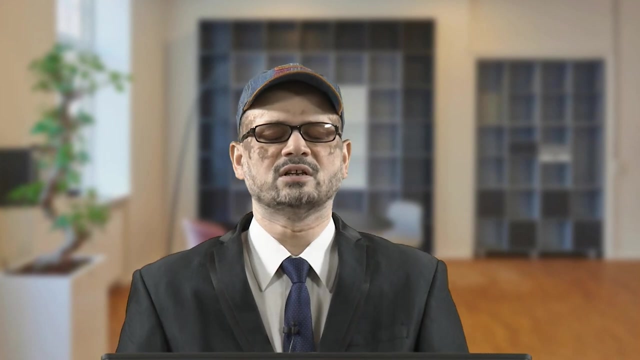 So we will have certain discussions in this lecture about those points. So coming to the introduction about that, So as we know that the phases in the material that may undergo changes as a function of temperature or pressure, So the change of that phase, normally what the material is undergoing, that will be known. 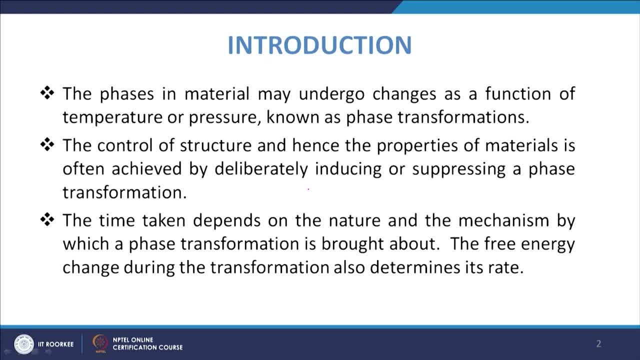 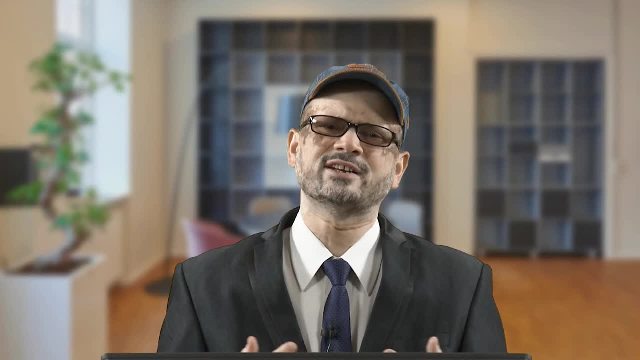 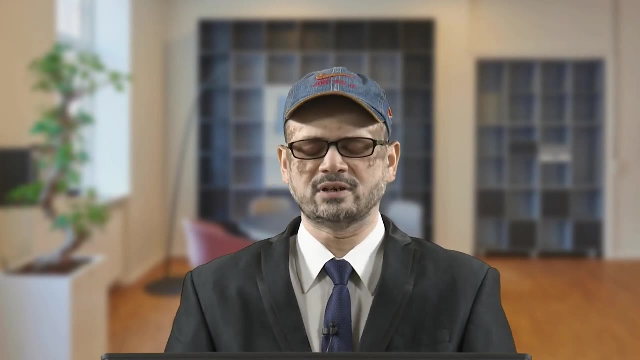 as the phase transformation. Okay, And the control of a structure, and hence the properties of material, is often achieved by deliberately inducing or suppressing the phase transformation. So, as we know that when there will be liquid to solid, suppose state transformation, Now, in that case we will have the light later on in this lecture that often occurs by the 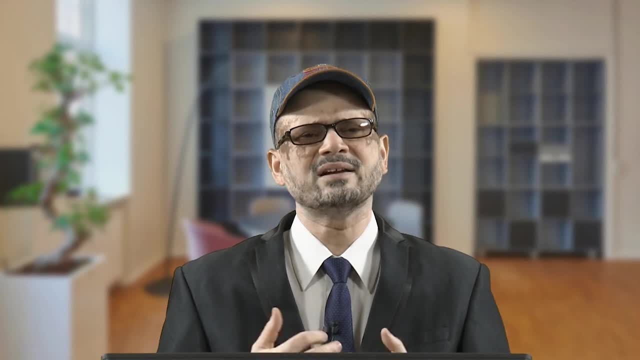 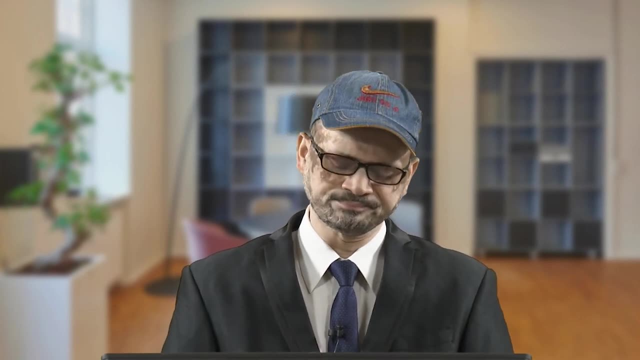 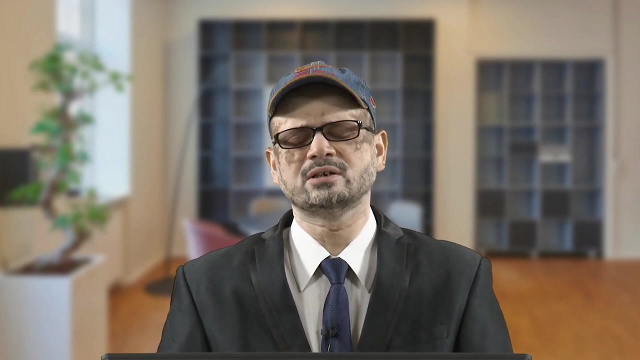 process of nucleation and growth. Okay, And basically that is what we call it. So the end result will be having certain structure and at micro level, that is known as microstructure. So now this type of microstructure which is achieved, or you know the properties which 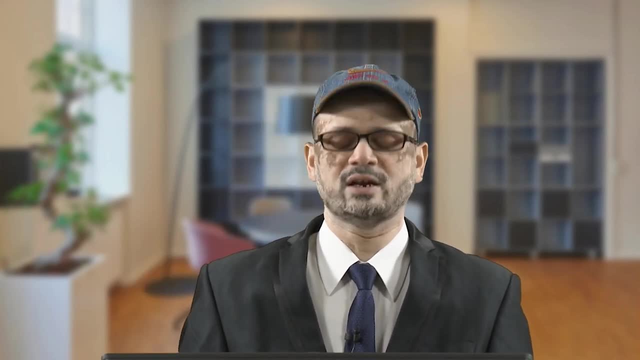 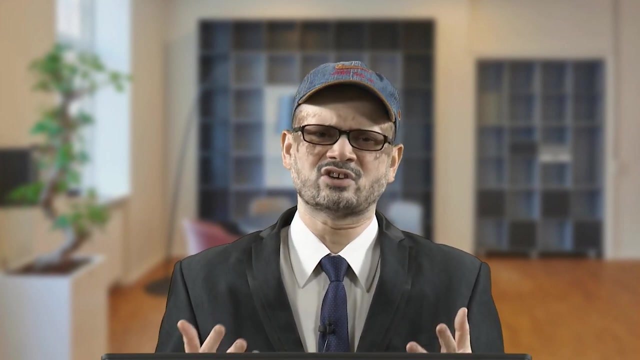 are the result of the type of microstructure you get. So that is basically, you know, achieved by deliberately inducing or suppressing the phase transformation. Okay, Okay. So phase transformation, if you allow it to happen in normal manner, then the structure may be something, and then if you try to alter it, you alter the rate of phase transformation. 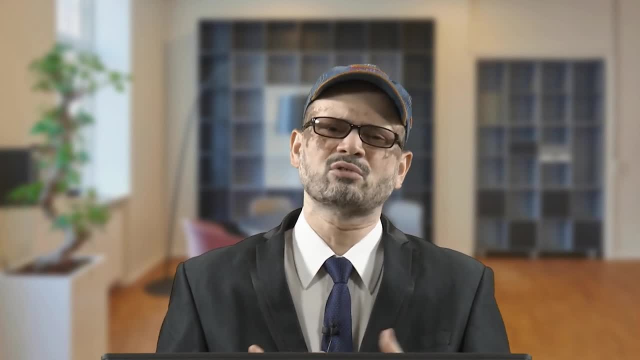 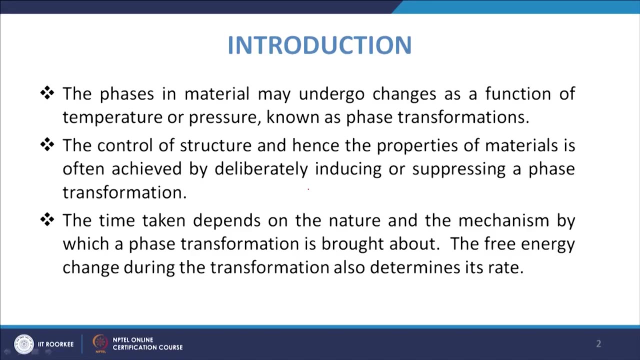 speed of transformation, then the, you know, structure will be different and associated properties will be different. So that is how? so the time taken? that will be depending upon the nature and the mechanism by which a phase transformation is brought about. So, by what mechanism that phase transformation is brought about, and the free energy change. 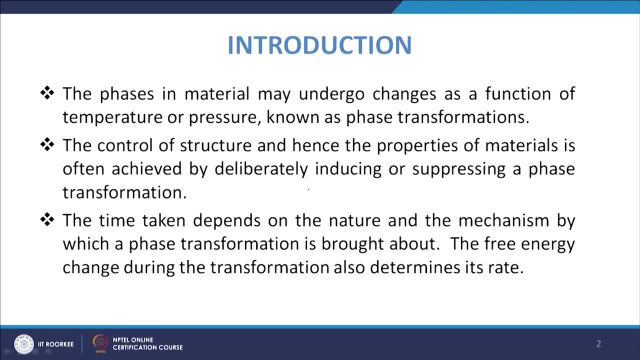 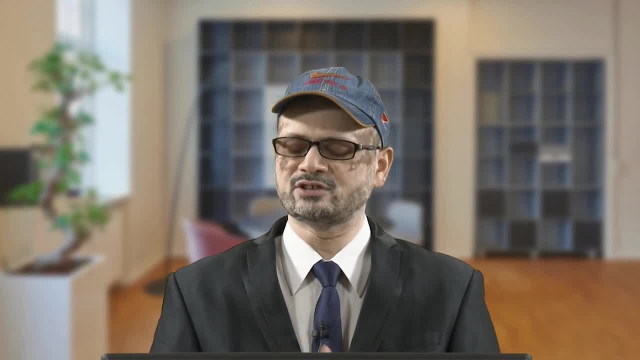 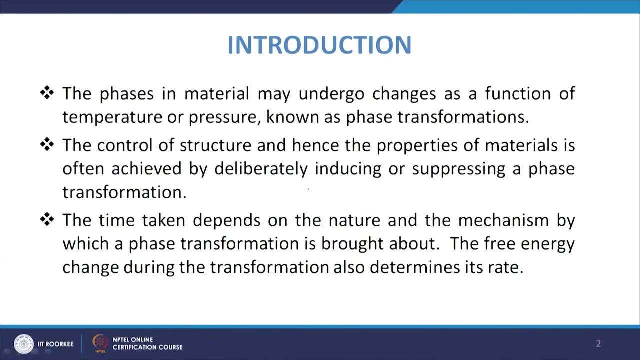 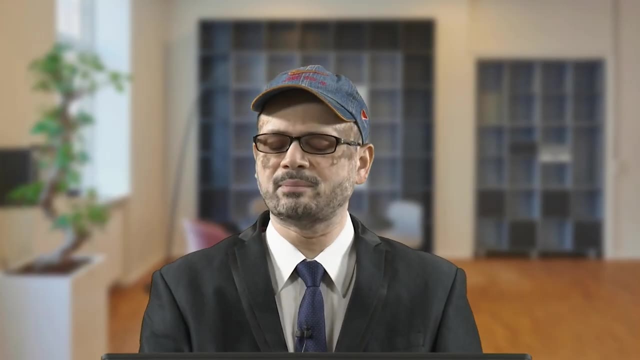 during the transformation also determines its rate. So basically we should know that the you know the free energy change which occurs, that basically will be determining the rate of phase transformation. So We will, We might have the understanding about you know the free energies you know because at 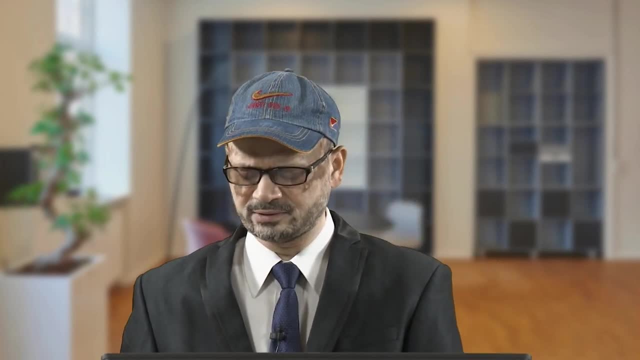 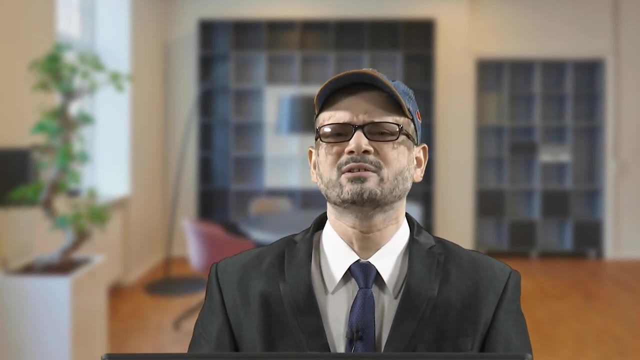 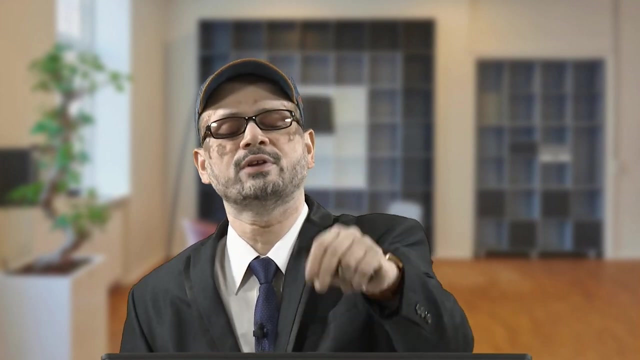 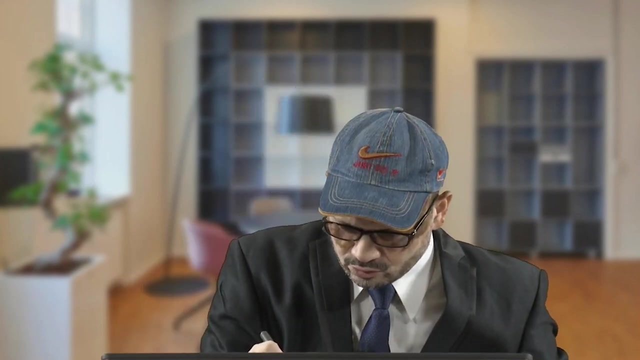 any. you know temperature or so at you know any material is in solid state or in liquid state, So that basically is governed by the free energy value. So if you talk about, say, free energy, So what we have might have, We might have this idea that if you talk about you know liquid to solid, you know transformation, 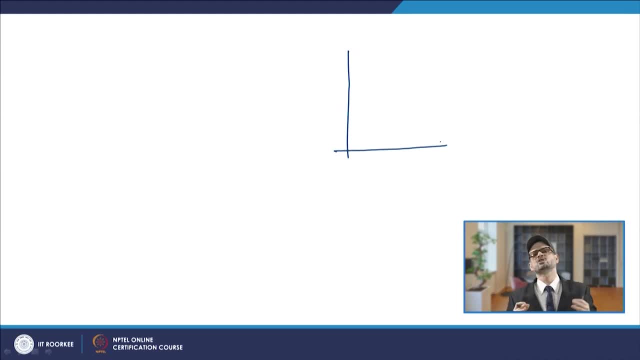 liquid. if the liquid is converting to crystal phase, Suppose beta crystal is being formed, So we can see that you know, if this is your free energy and so this is, you know, G, And if you take this as temperature, So any material, if it is in any phase or state at any temperature, it is all governed by the 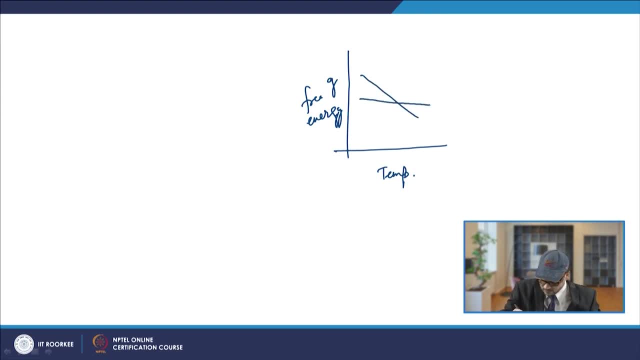 you know phase free energy values. So the free energy values go like this: you know this is your equilibrium temperature, or you can have the. so that is normally the melting temperature Now, if you do know that. So, So this is after a melting temperature. 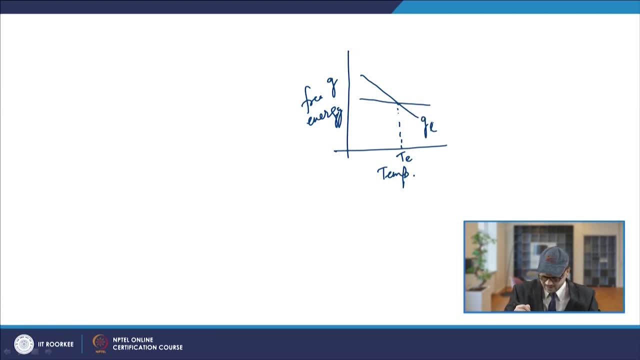 So this is basically the free energy for the liquid phase and this is free energy for the solid phase. suppose solid crystal B is beta. So in that case your below the equilibrium temperature. you see that this line is for the free energy of the solid phase or beta. 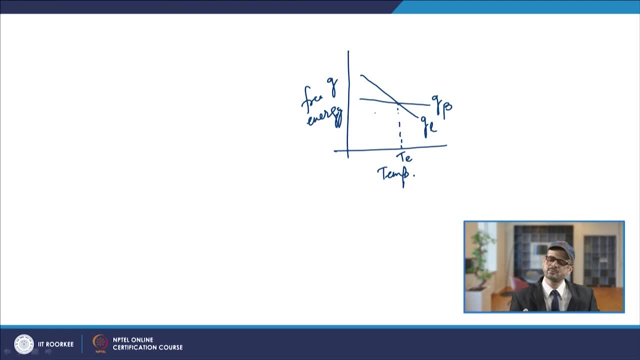 So below the, this equilibrium temperature, This free energy value of beta that is solid form is less, So material exists in solid state. And once you increase the temperature after this equilibrium temperature or melting temperature, So in that case you know the liquid state or liquid phase has the higher, you know you. 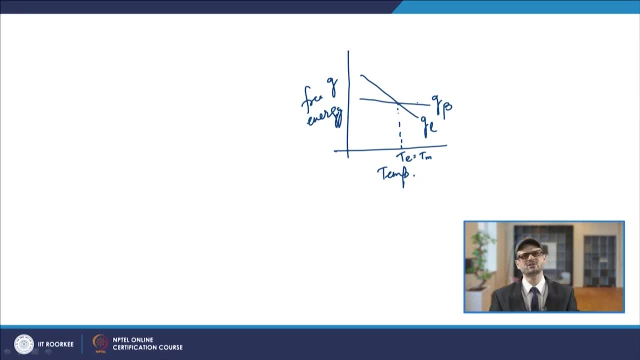 know, lower free energy value. So it comes into liquid states. That is how The material exists, either in the form of liquid or solid phase. and you know we can say that whenever any transformation has to occur. you know So what is being said. 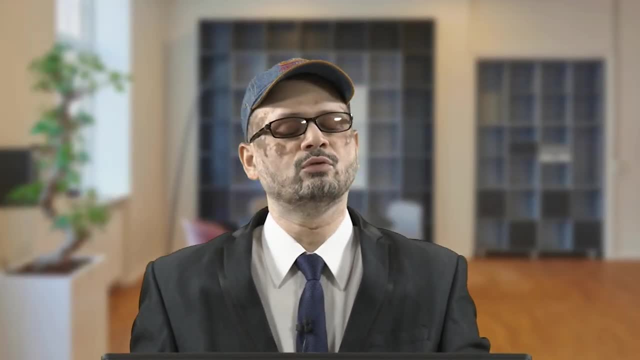 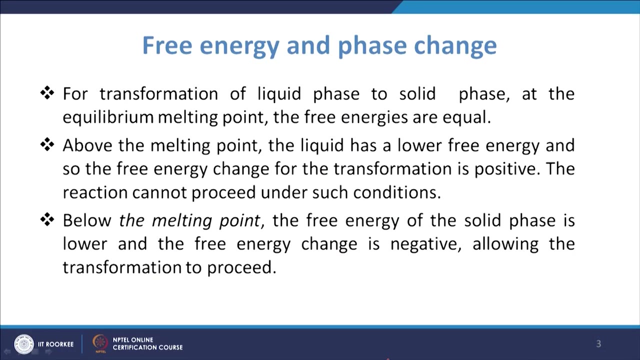 So if you go to our next slide, So for a transformation of liquid phase to solid phase at the equilibrium melting point, The free energies are equal. So that is what it is clear. We have seen, that when the curves are meeting at the equilibrium temperature or the melting, 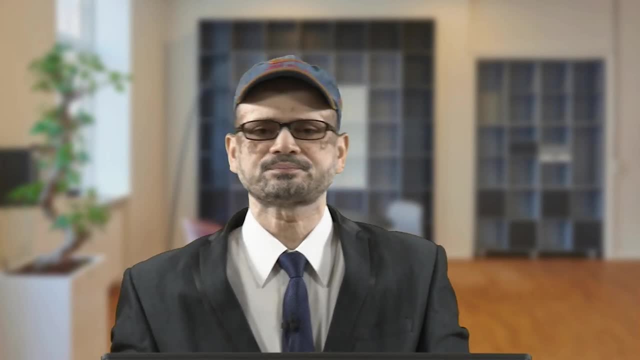 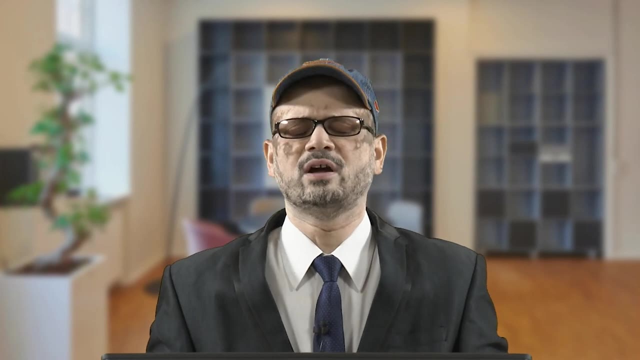 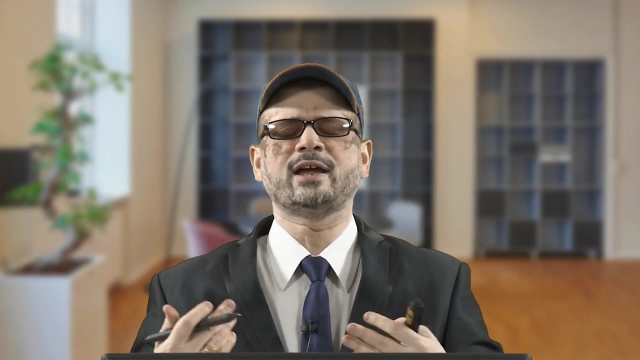 point, temperature. At that point the free energy value of the liquid as well as the solid phase. they are equal and there will be no transformation occurring because the solid and liquid, both are existing in equilibrium there. Now, if you take the temperature above the, you know melting point. 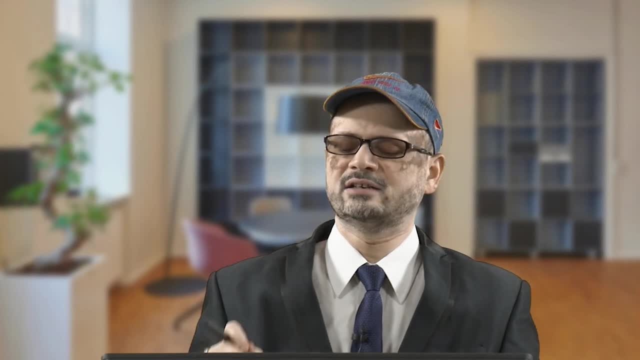 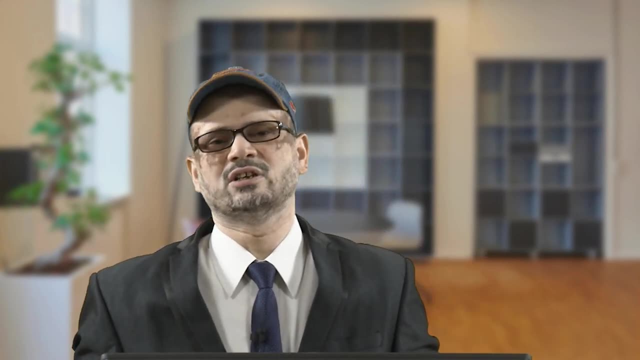 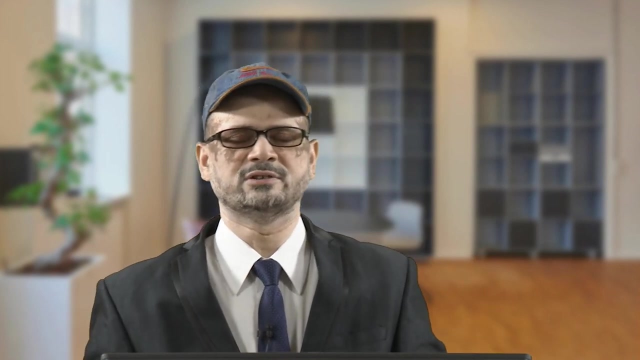 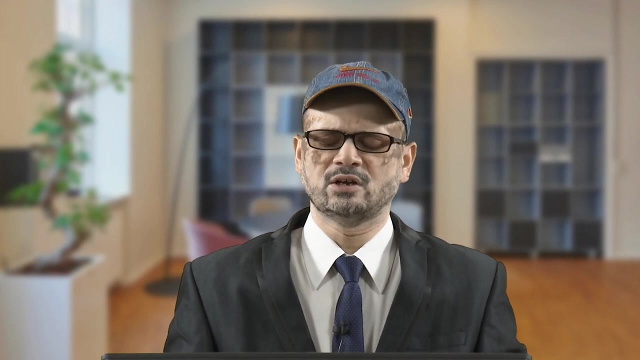 Then what we have seen? that there is liquid which has the lower free energy And so the free energy change for the transformation is positive, Certainly because that change will be positive and so there will be no transformation. you know, going on, then, if you take the, you know, if you take the temperature below the melting, 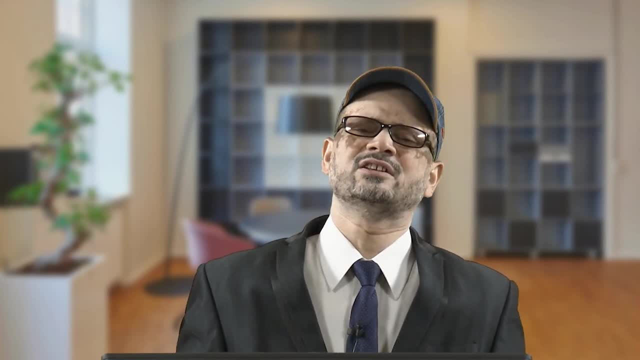 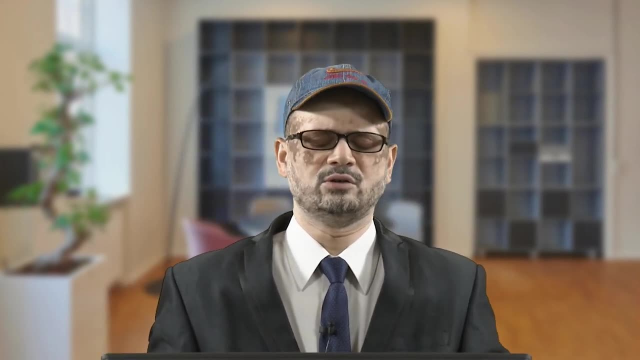 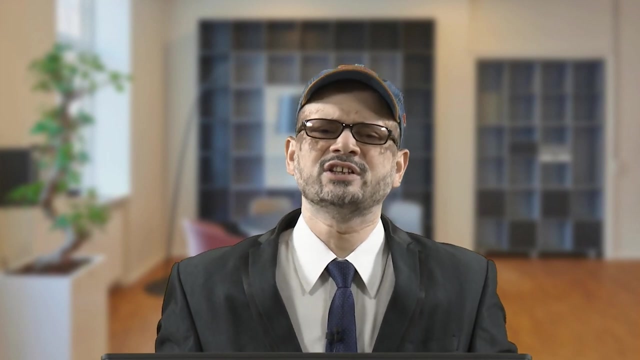 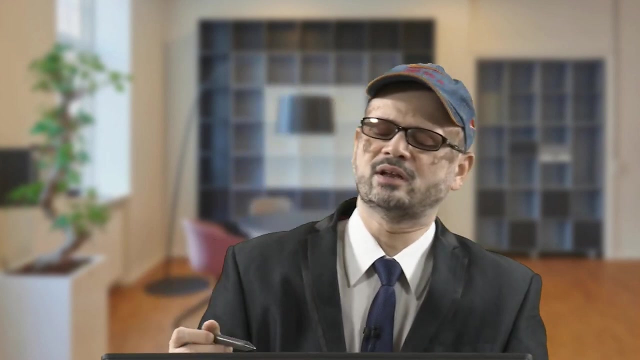 point Ok, the free energy change will be lower because the liquid will have to come to, you know, solid values. If you take the free energy change values, you know that in that case. so if you take this, this is your liquid value. so if you have to change from liquid to solid and if 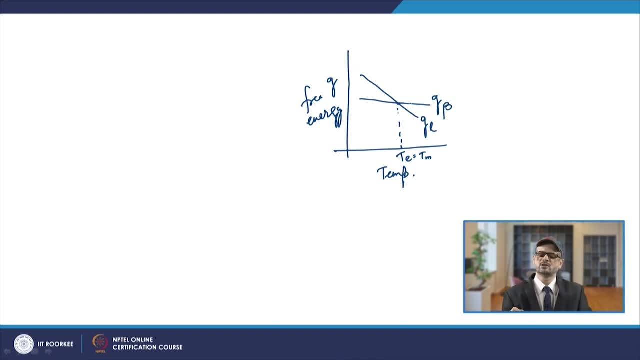 you take, you know so that free energy change value will be positive, So there will be no transformation after this temperature, while if you take the temperature below, since the free energy value of the- you know- solid phase is less than the liquid, So the free energy change value is negative, 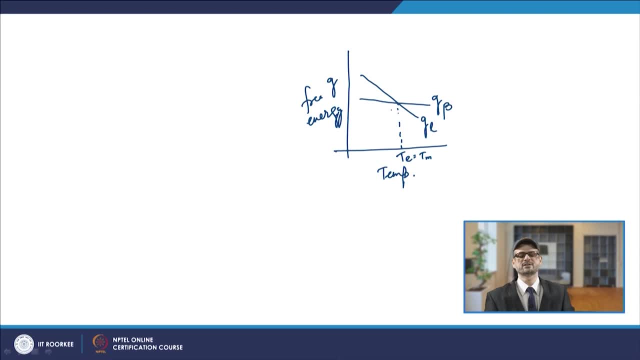 So that is why, once you have the temperature less than the melting temperature, then there will be transformation Proceeding from liquid state to solid state, and you know that is the essential mechanism of having the phase. at any temperature. what, in what phase the material will exist. 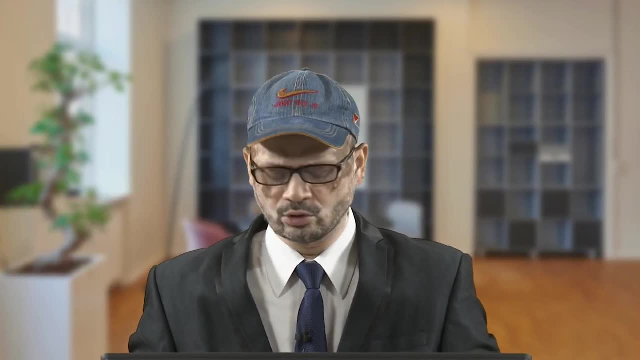 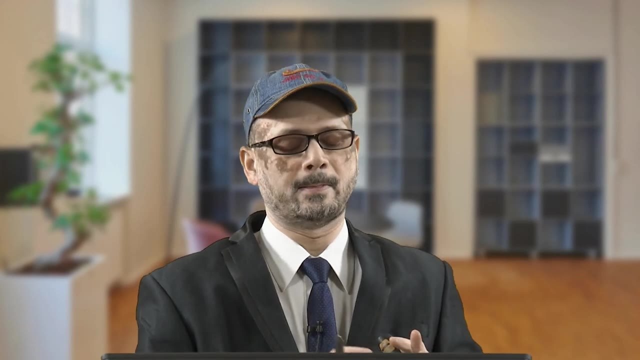 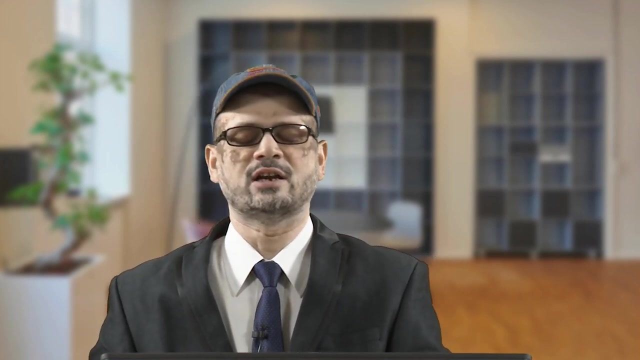 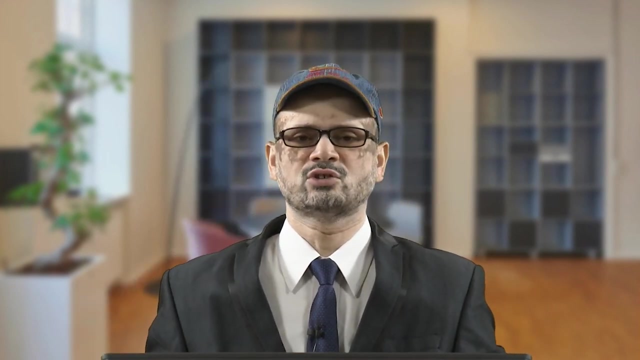 So now, what we need to know, that this mechanism, by which you know this Okay- Transformation has to occur, So that is, by the mechanism of nucleation and growth. So when the magnitude of this free energy change is very small, the reaction proceeds very slowly. 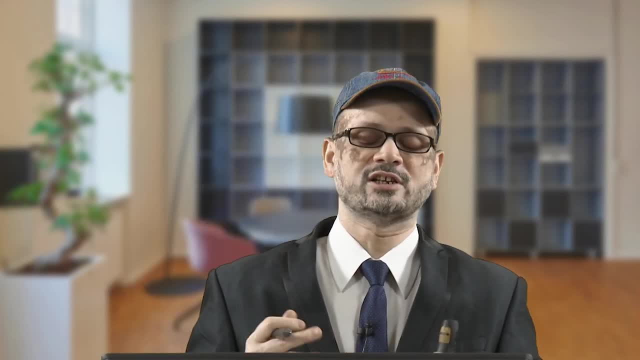 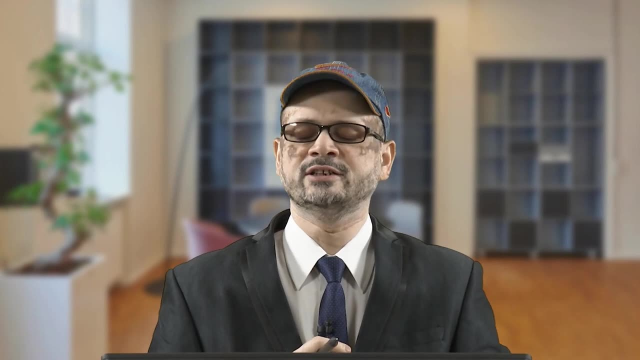 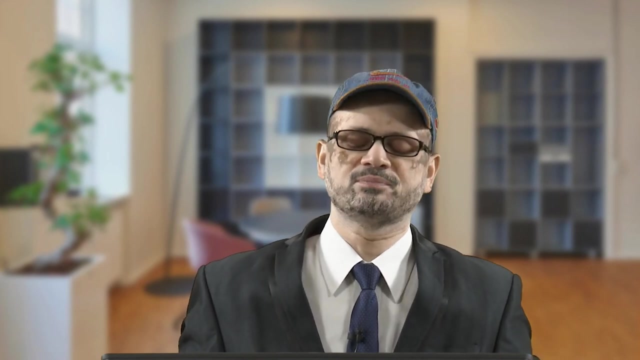 If you talk about the scale of transforms and time scale changes of the transformation, So the magnitude of the free energy change what we have seen. if this is very small, then reaction will proceed very slowly And with a large super cooling below the equilibrium melting temperature. the magnitude of free energy. change will be large If you take the equilibrium melting temperature and from there if you have the temperature quite less, so if the degree of super cooling is more or under cooling is more, that is difference between that equilibrium melting temperature and the temperature which we are talking about. 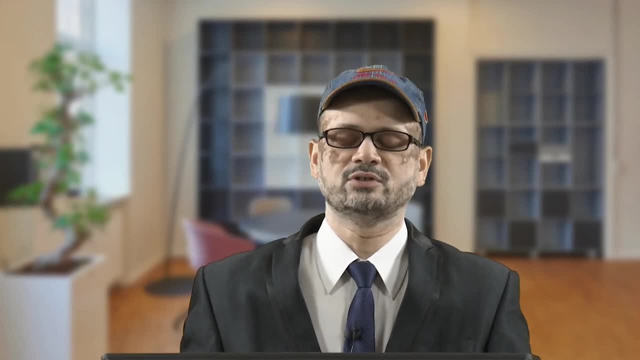 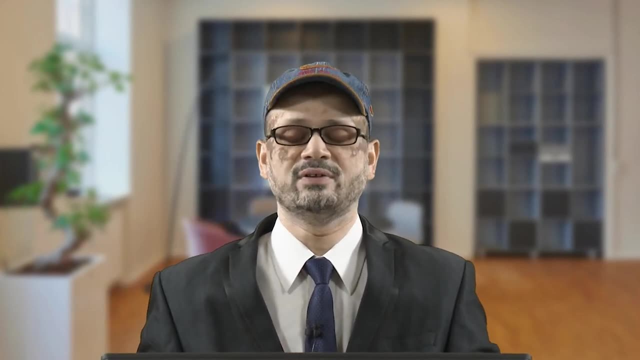 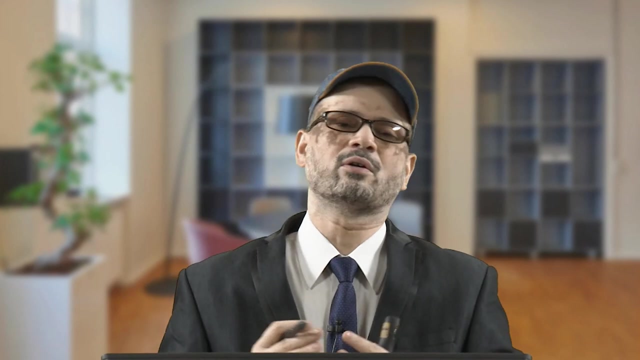 In that case You will have very fast, you know, transformation. So and if it is very small, in that case the reaction will proceed very, very slowly. So you will have many kind of, you know, if you talk about the qualitatively the transformation scales. 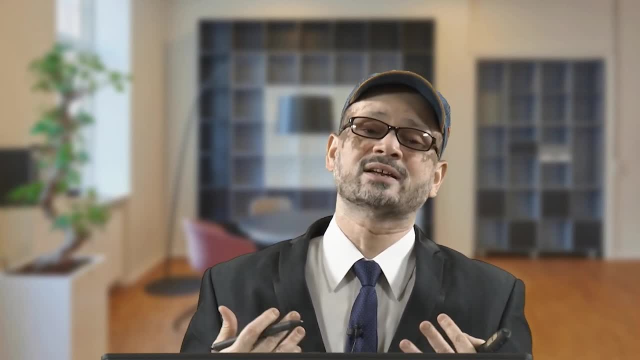 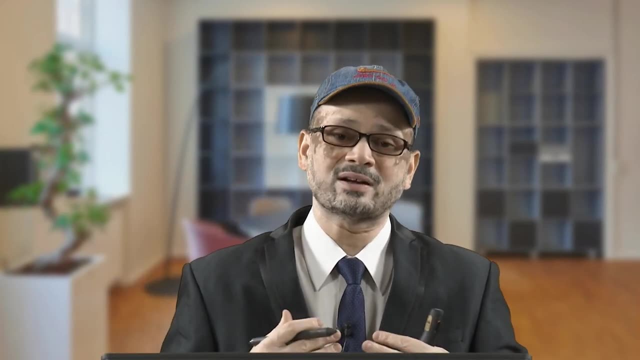 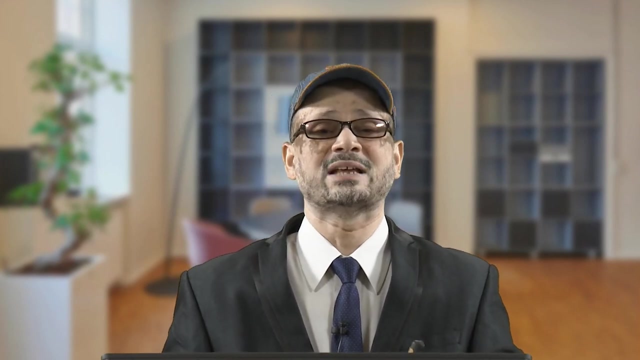 In that case, if it may take time from milliseconds to years, and that will be representing, you know, the The also that what kind of transformation it is, whether it is very fast, whether it is fast, moderately fast, or whether it is slow or it is extremely slow. 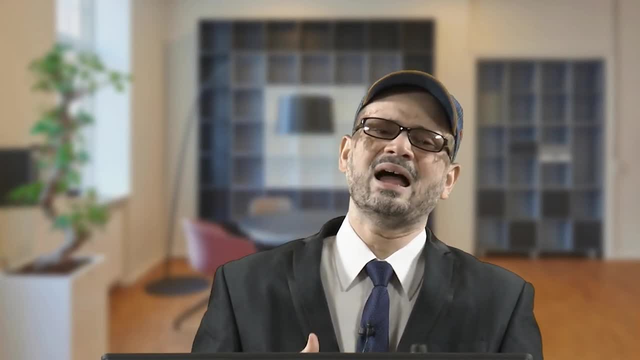 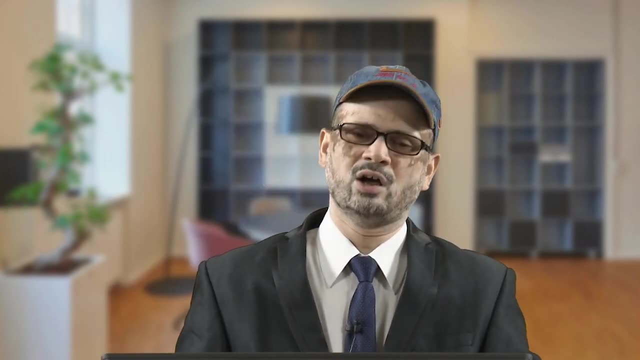 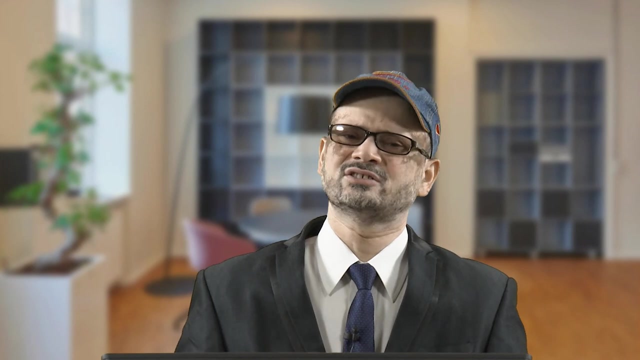 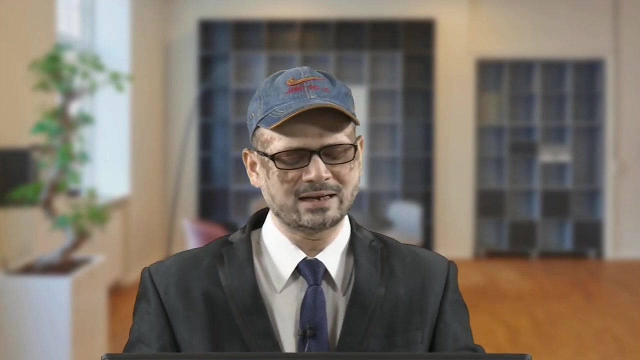 And depending upon that, you know, you will have also the concept of suppressibility of these, you know, transformations. So when in the transformation is extremely fast, it is occurring in the term of microseconds, It cannot be, You know, suppress, so it is insuppressible, whereas below that, you know, if it is very. 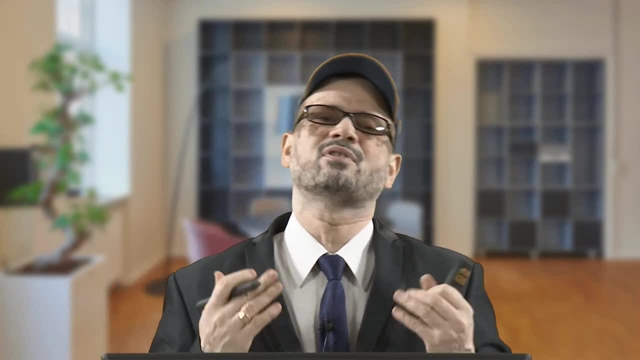 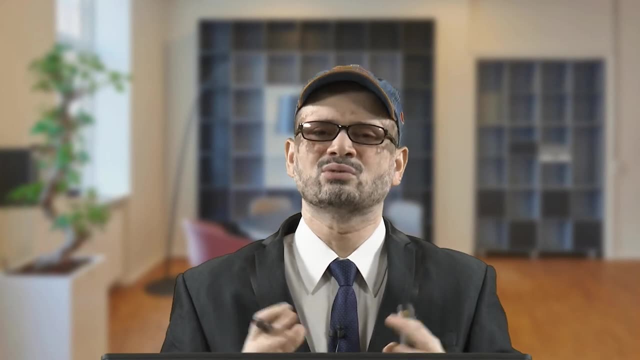 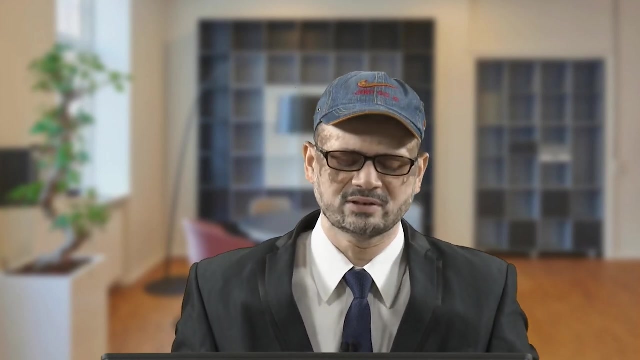 fast. if the if that takes time, maybe from milliseconds to seconds, in that case it may be suppressed by very, very large cooling and then it is suppressible in the normal case when you have slow transformations or you have fast transformation, that way it can be suppressed. 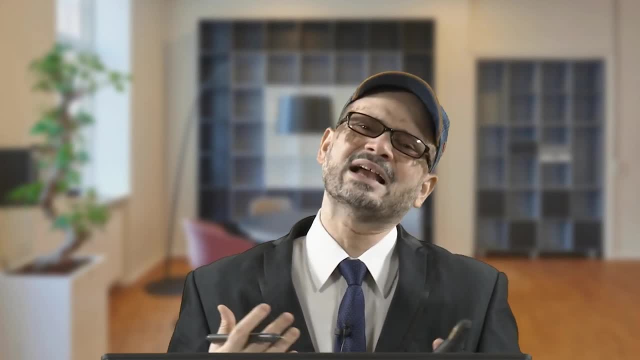 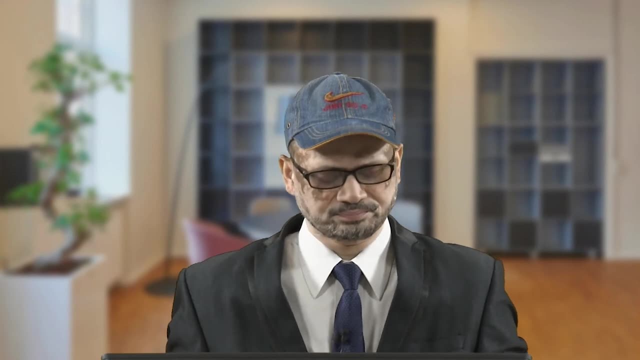 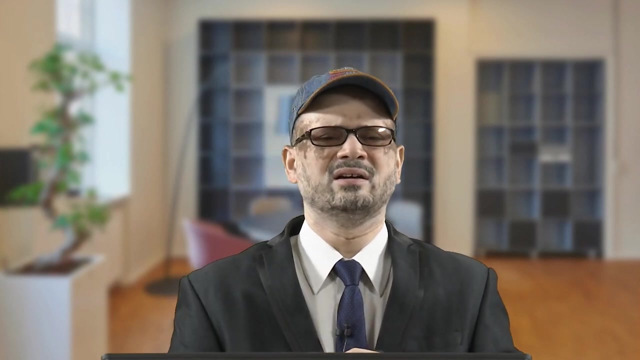 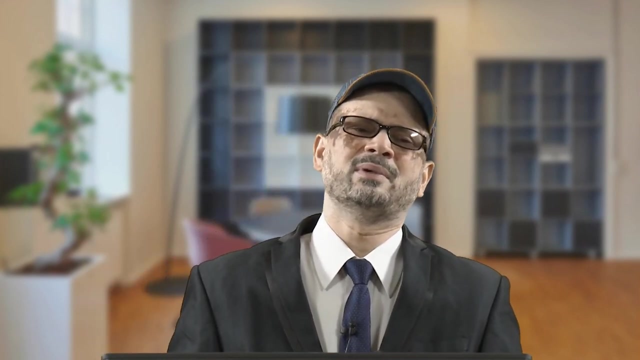 And You know, when it is extremely slow, Then in that case the suppressibility is normally not possible. So in that case, basically, transformation is virtually impossible because the you know that it is extremely slow in nature. So you have many, you know methods to go. you must have seen that in normal case you are. 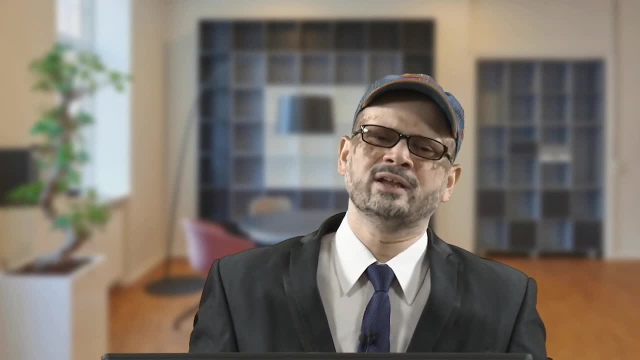 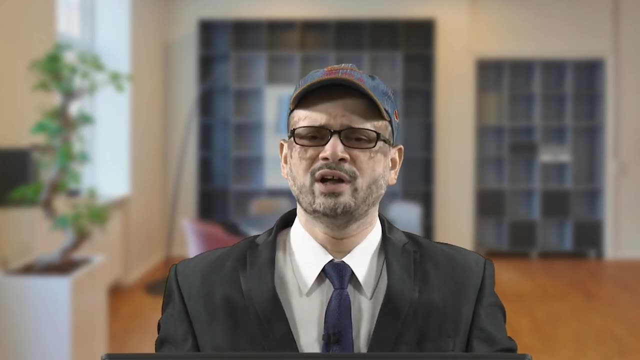 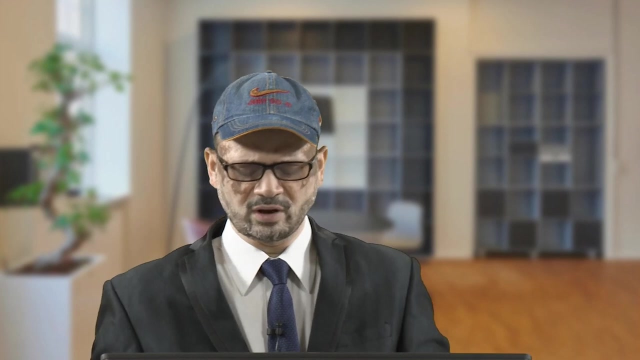 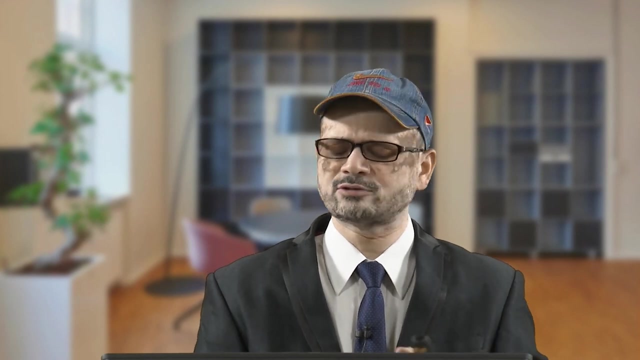 cooling in the air, Or, You know, cooling in the water. You go further to increase that by cooling in the oil or brine solution or so, And you have splat cooling, which is very, extremely high cooling rate, or so Now we will talk about you know the. so the next point which is important is that transformation. 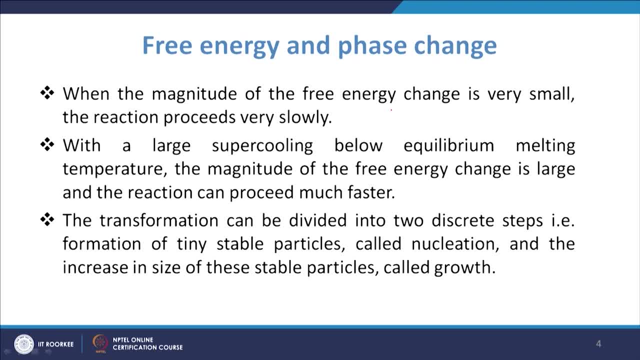 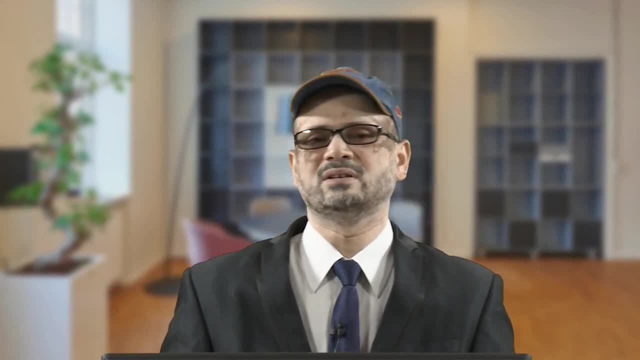 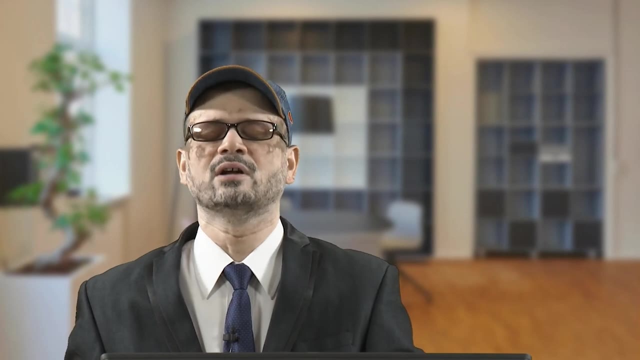 is divided into two discrete phases, And these two discrete phases are that you have The Formation of tiny, stable particles, that is known as nuclei, and then further you know the growth of these particles, so that is known as growth. So with that mechanism basically, your transformation is basically complete. you have transformation. 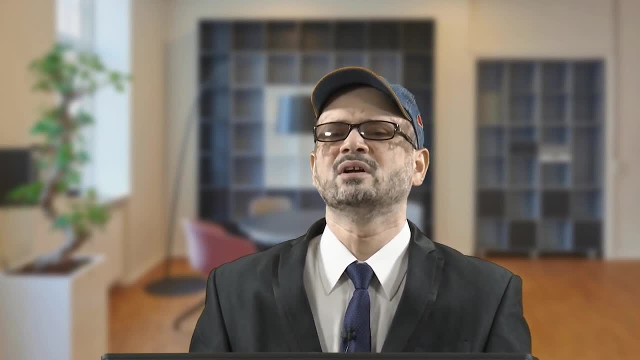 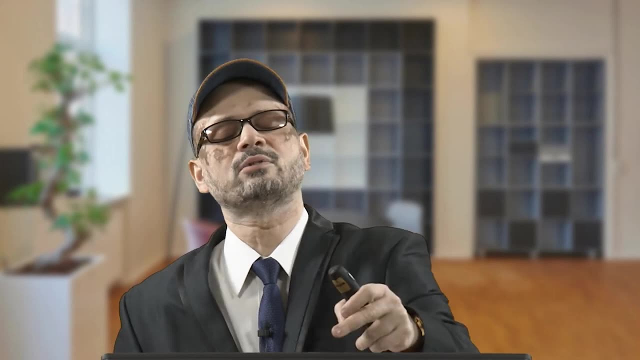 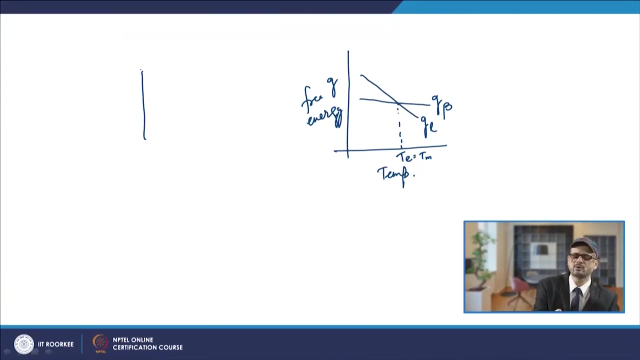 is complete by the mechanism of. you know nucleation and growth And You have certain understanding about the concept of nucleation and growth. So, as you know that if you have a liquid domain, your domain filled with liquid, in that case you have all, everywhere you have liquid. 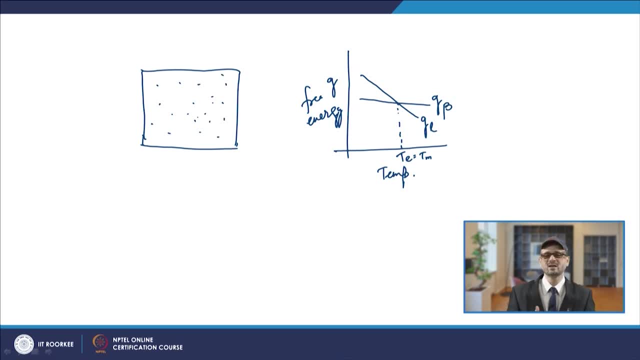 Now, when the temperature will come down in that case- and it will come down below the equilibrium melting temperature- then there will be transformation started from liquid to solid phase. Now, as we know that, when the solid crystal has to come out of the liquid phase, So that will be by the birth of a new phase. 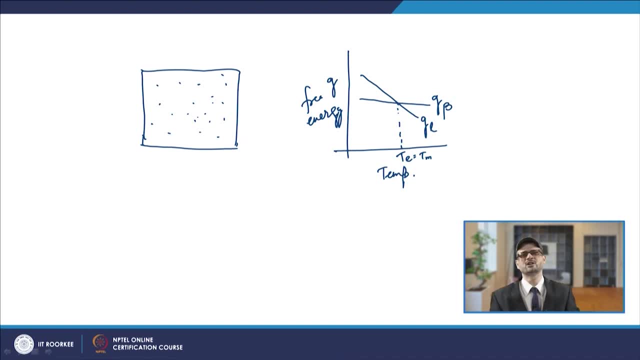 Now, any new phase, if it is created, you know it requires energy to be supplied, So that energy, you know it has, you know to be supplied during the transformation. and if you talk about So it is very small, tiny particle, in that case the for, and if you assume the particle, 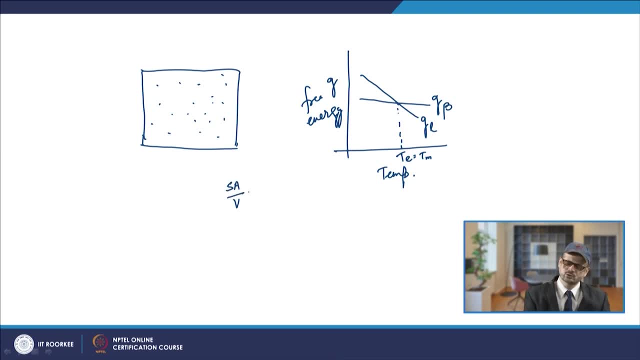 to be spherical, then the surface area by volume ratio that becomes if you take the spherical particle, so it will be 4 pi r square divided by basically 4 by 3 pi r cube, So it will be coming as 3 by r. so basically when you have very, very small r. so if r will 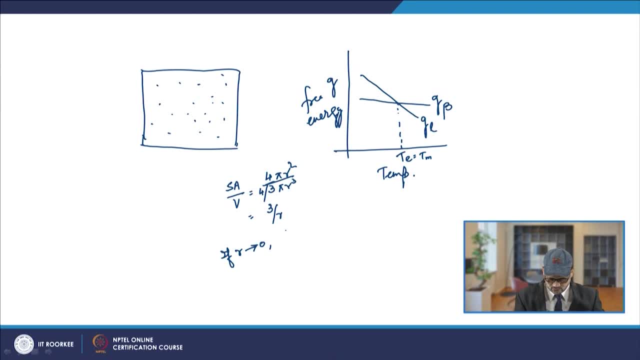 be approaching towards 0. So this ratio S A by V is moving towards infinity, very, very large. So initially it will be preventing the formation of new interface, you know. so that is why, But then, as this r if you are at one point of time, this r if it is more, in that case, 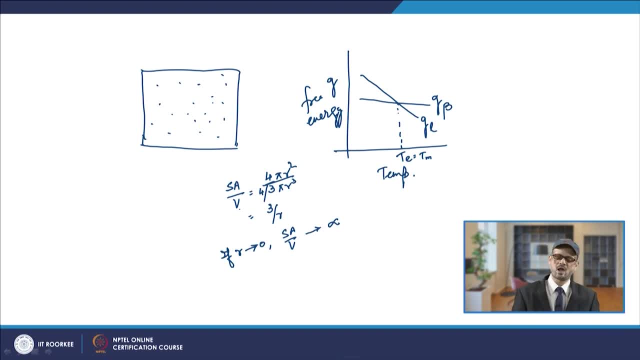 this, you know, as the r goes on increasing. 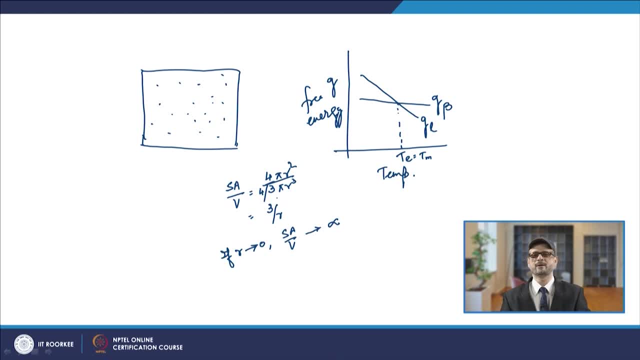 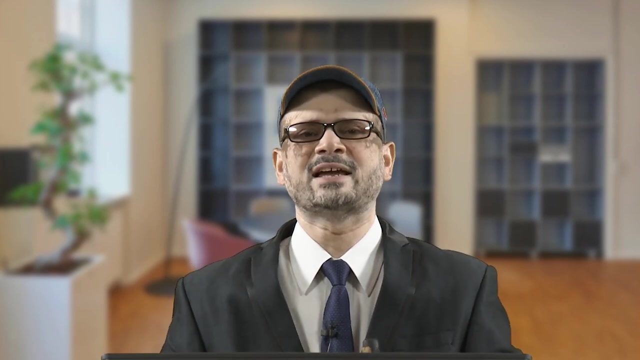 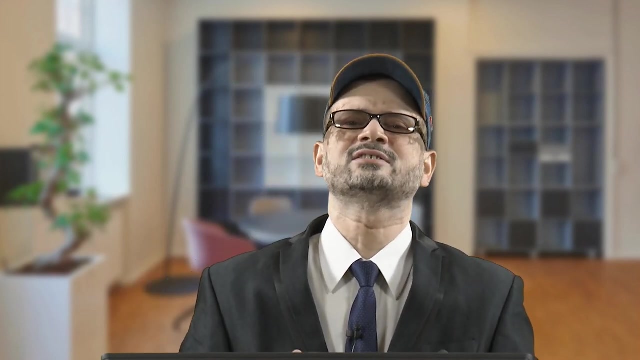 So the thing is that in the case of, you know, homogeneous nucleation, your probability of nucleation at all the sites inside the domain is identical, And in heterogeneous nucleation the probability of nucleation at preferred sites are more, so at certain sites they are more. 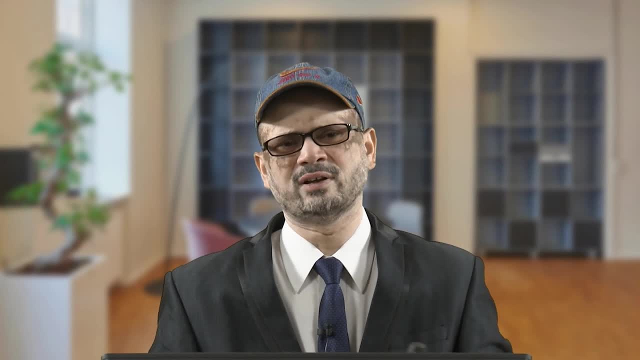 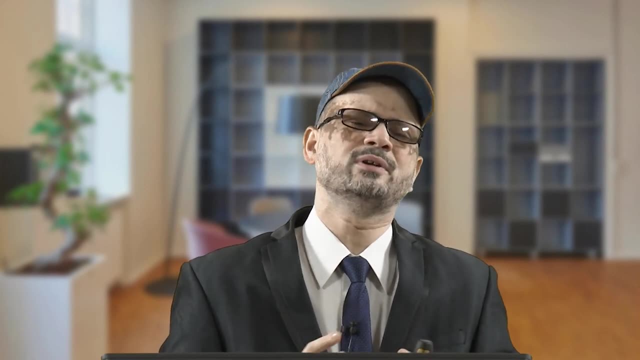 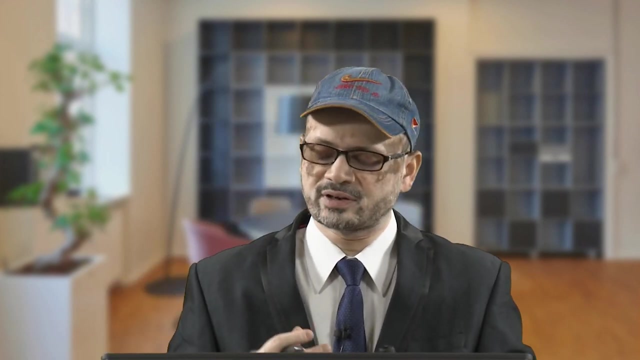 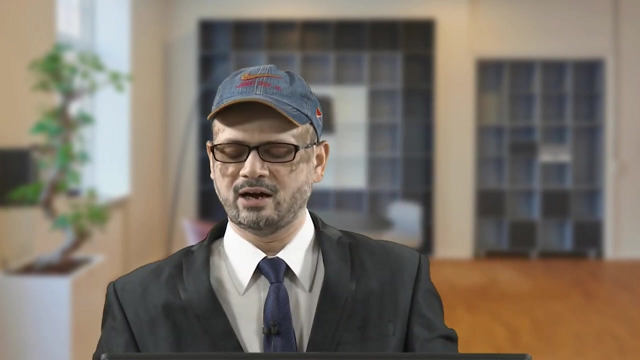 So in normal case, when you have a domain and you do not have any preferred, you know nucleation sites so that will be homogeneous nucleation. If you assume that to be homogeneous for a homogeneous nucleation, you know case. so if you take the delta F as the free energy change, so if delta F is the free energy change, because 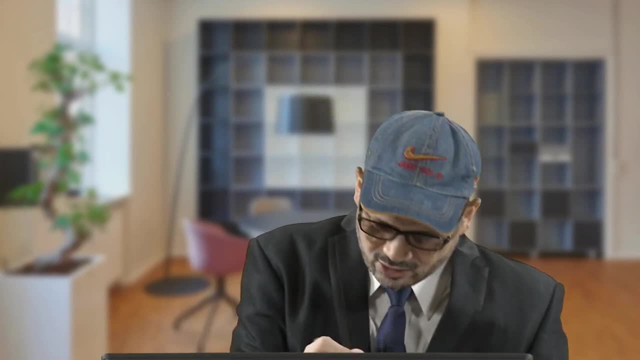 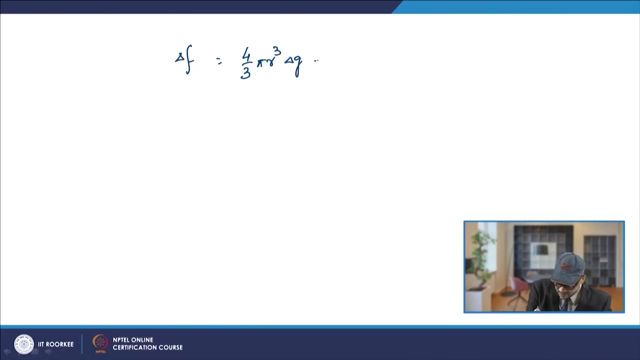 of the formation of a new spherical particle. so it will be 4 by 3 pi r cube and this will be delta g plus 4 pi r square and gamma. So basically, a one will be positive term, another will be negative term. so that is. 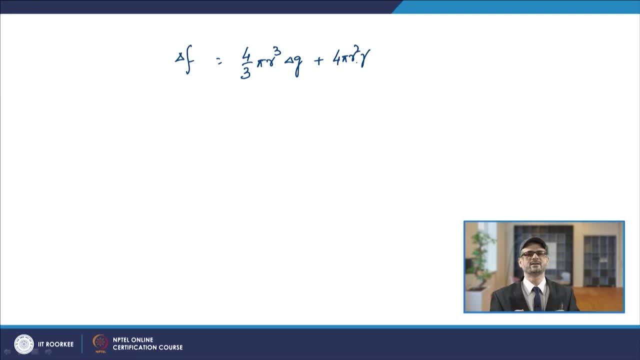 your volume free energy, and we know that it has to be negative, you know, for the transformation to proceed. So where this? so that is why you have r as the radius of particle and you have delta g as the Gibbs free energy change per unit volume. 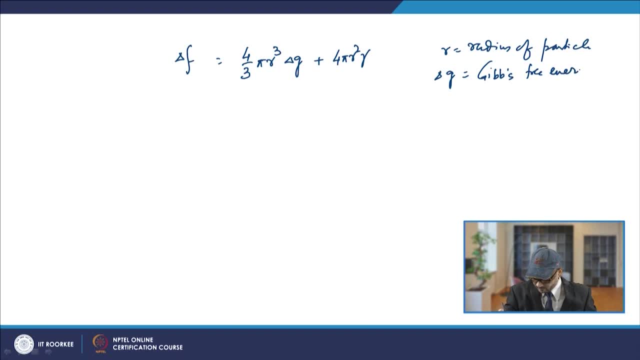 And if you talk about the gamma, so it is surface energy per unit area Of interface separating the parent and product phase. So you know that this will be positive. you know term and this will be negative term and you will have Free energy. you know curve and that curve, basically what happens, that initially, when it is very small value of r, then this value will have very large value and positive value. And when, as the r, you know, as the radius of that nuclei, increases, in that case you will have So, ultimately, as the r increases, this term is termed as free energy. 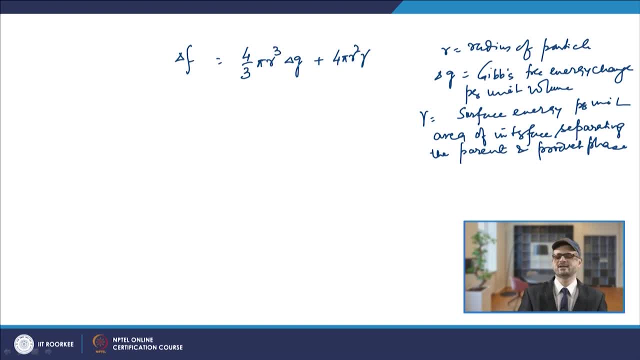 And then your resultant delta f curve will go on decreasing. so you will have a point at which, after which it starts decreasing, and that is the point from where the transformation formation is supposed to start. now. so for getting that point, so what happens that if you talk about the, you know free energy, those values. so if you take this as the, you know 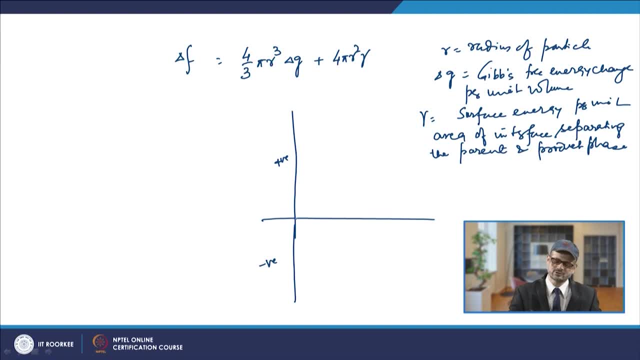 positive and this as the negative values. So what happens initially when you are, you know, varies. for a small, very small value, this is going towards very high infinity. but then, once you, and if you take this value, normally it goes like this: so this will be 4 by 3 pi r cube delta g plus 4 pi r square gamma for 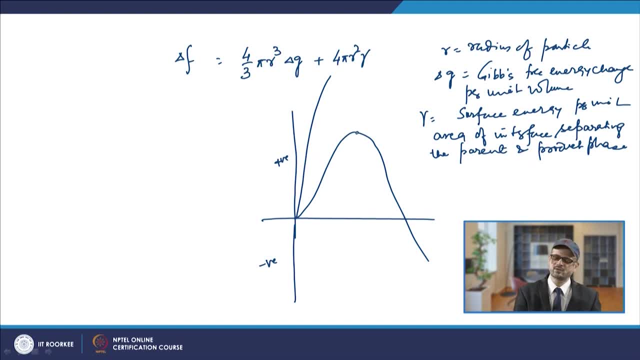 this side. Now, this is the point you know. 4. From where it starts going on decreasing. So, for getting this point, what we do is d by dr of delta f, we are doing it, equating it to 0 for getting this value of r. 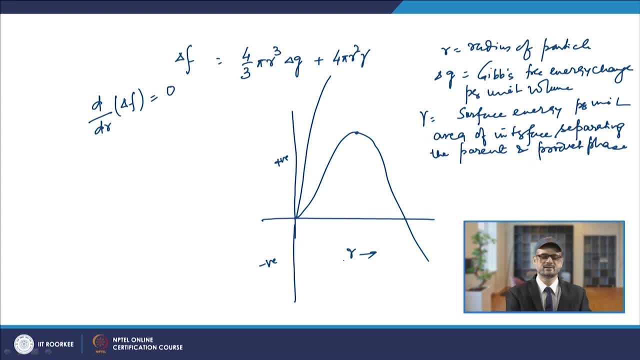 So this is r basically and this is delta f. So if you do that we get basically the, so for that we are calling it as r star 4. And this will be minus 2 gamma by delta g, so this is known as the critical radius in. 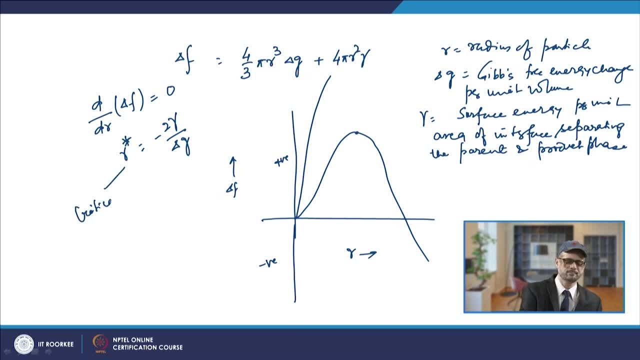 this case and of the nuclei, and for this the delta f star also, it is critical value. if you put these values into this expression: 5.. So it will be 16 by 3 pi gamma cube by delta f 6.. So this is what the value you are getting, you know, for the delta f star. you know values. 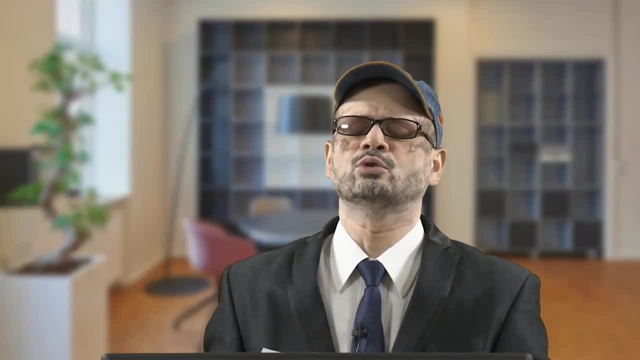 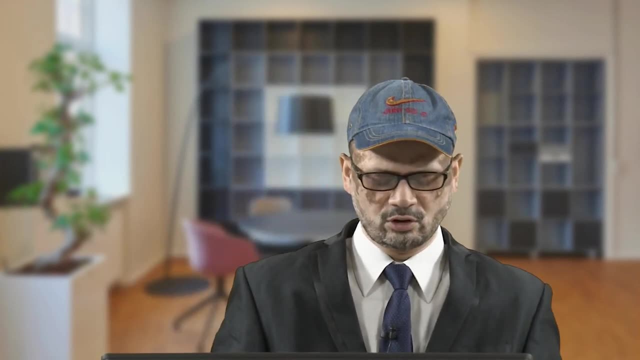 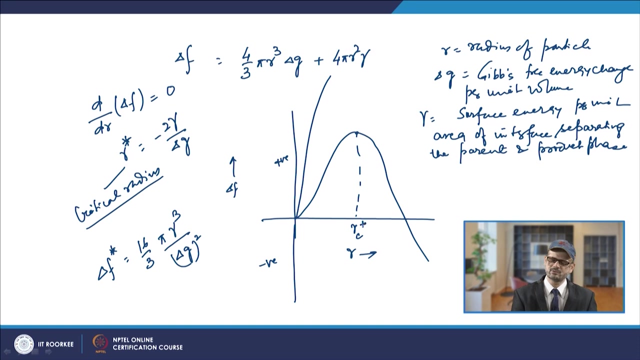 Now you can have another also. you know expressions for these delta f star, or for the transformation, also 7.. Now if the radius, So this will be your critical radius, 8. And that will be known as r c a star. Now, if the radius of the particle is below this line, I mean towards the left in that 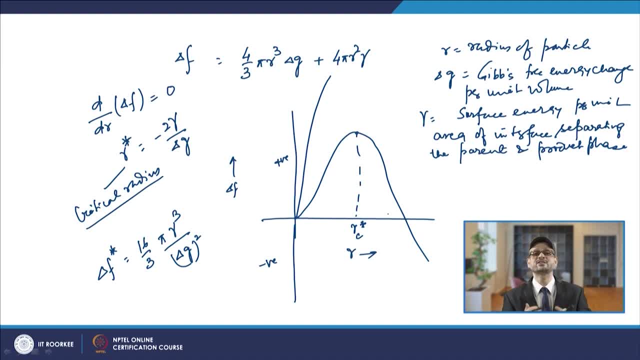 case it is known as embryo, and if it is after that, it is said to be nucleated. So then that is basically the nuclei. there are- there are another, also expressions for liquid, to suppose the beta 9.. So that is basically the nuclei. 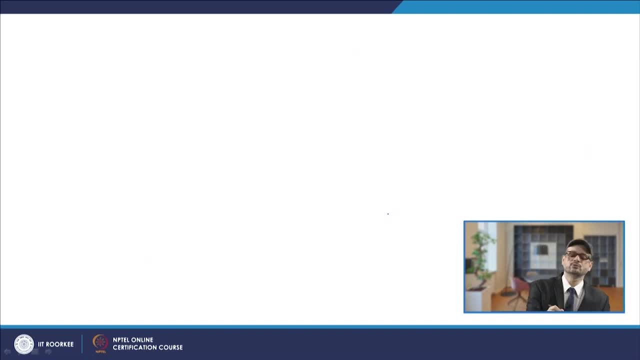 10. So that is the transformation. 11. So if you talk about for liquid to beta transformation, so you have another, you know, simplified relationship that is that holds good. is delta g equal to delta h into Tm minus T upon Tm? 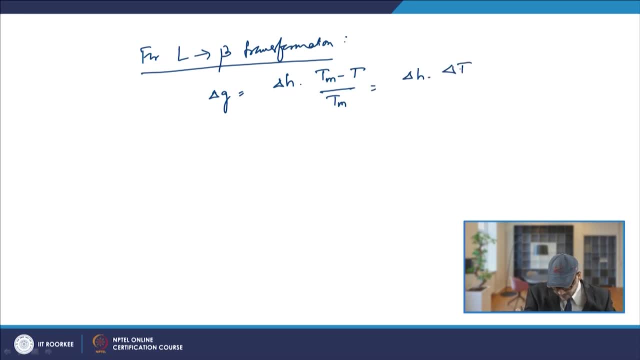 So basically it will be delta h into delta T upon Tm 12.. So basically delta h is you know that it is enthalpy change, or we also known as know it as heat of reaction. per unit volume of the product, heat of reaction. 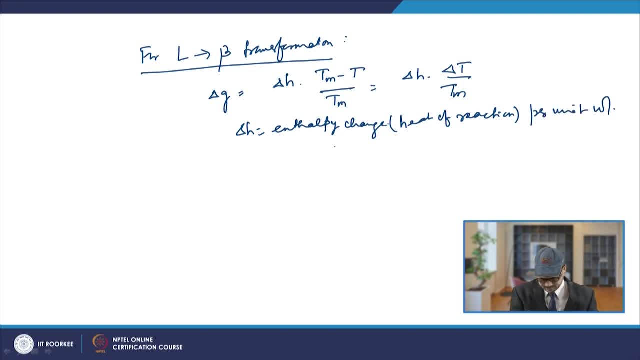 So that is per unit volume of the product 13. And it is independent of temperature: 14.. So that is per unit volume of the product 15. So it is independent of temperature. and Tm is the equilibrium melting point, and at Tm 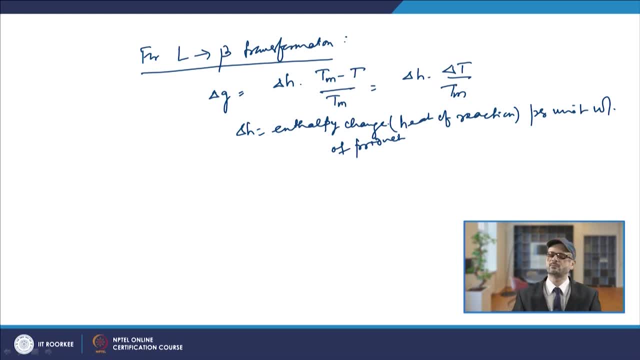 basically this: delta g certainly if you talk about at Tm, so it will be delta T is 0, so delta g becomes 0. 16.. Now if you use this formula, so you get the expression for delta f star, that will be 16. 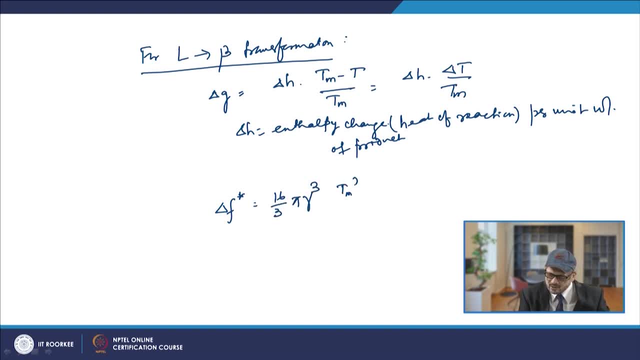 by 3 pi gamma cube and Tm square upon delta h square and delta Tm 17.. So this is another expression you know for which, by which you can get the value of delta f star, that is your, this barrier, now you know, and that will basically be affecting your. 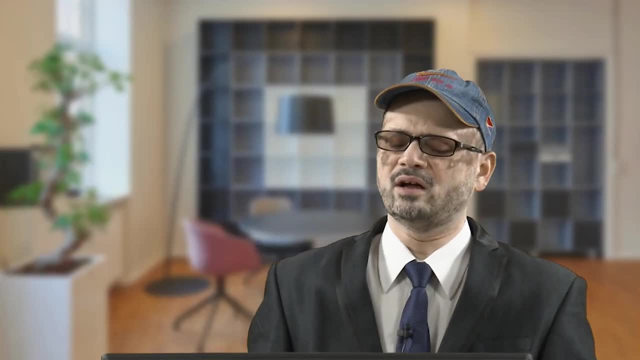 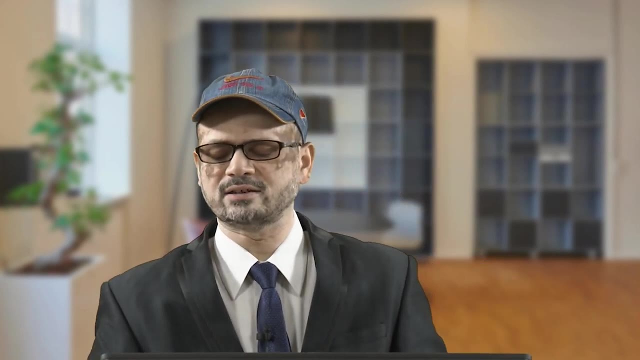 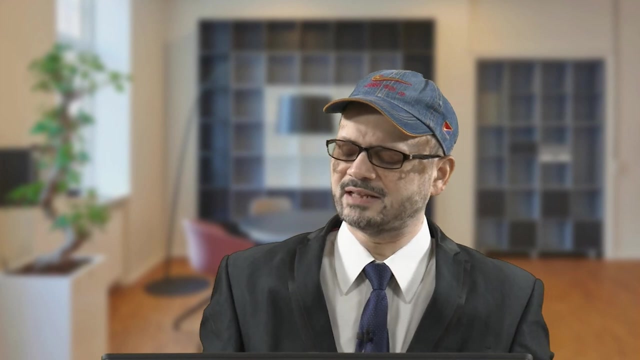 nucleation process. Now further. so that will be just you know. this is this gives you the concept of delta f, star 18.. So this is that when you have, you know, you know the number of critical sized particles that basically can be estimated using the Max Boltzmann statistics. 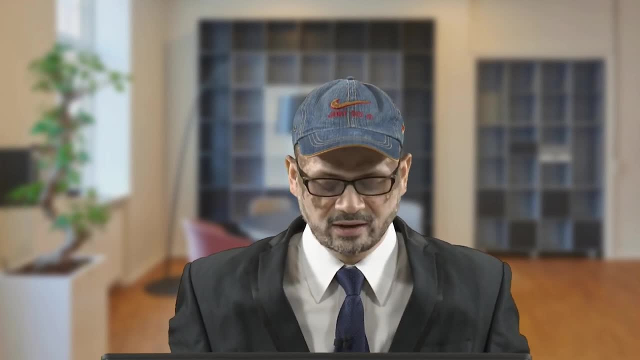 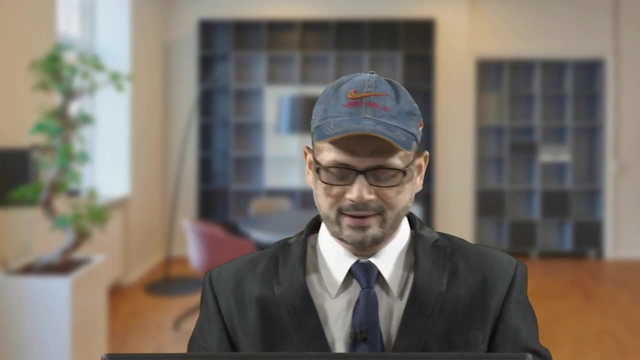 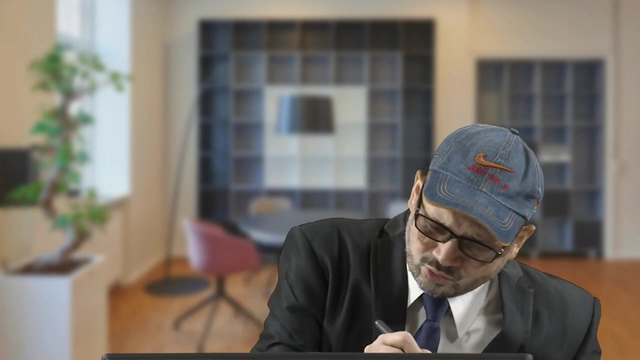 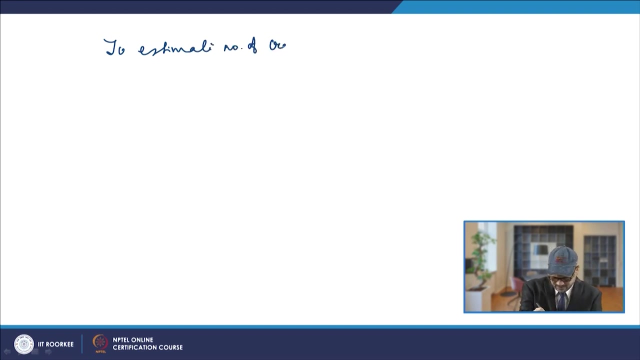 So that statistics concept is used and for from that Max Boltzmann statistics. if you try to find the, you know the number of these particles, So if the 19. So you have to estimate number of. you know critical sized particles, So for that the Max Boltzmann statistics is used. 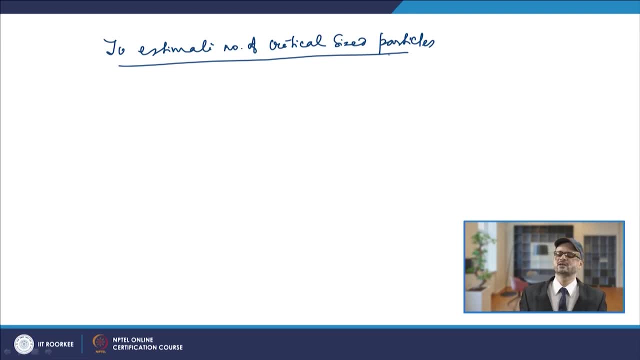 So how? what will be the number of critical sized particles in the apparent phase? So if Nt is the, you know- total number of particles per unit, volume 20.. So you have to estimate Volume Of parent phase. in that case, if you have to find the number of critical sized particles, 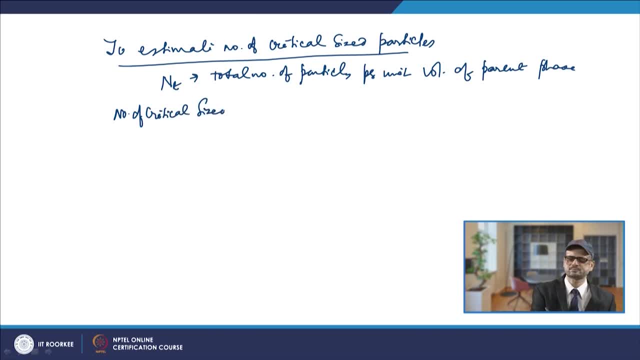 So number of critical sized particles that, if you, you know, denote by N star, so it will be denoted by Nt And this will be exponential of minus delta, f 21.. Star Divided by RT, So this will be the value of the number of critical sized particles and the process of 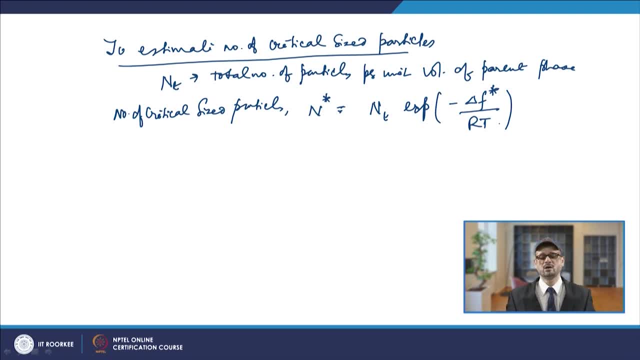 nucleation is that, you know, is that step of process when this, this critical sized- you know- particle, becomes supercritical, So that will be By jumping off one of atom, the atom from the parent phase to the product phase, so that basically will be make it supercritical. you have a critical sized particle and then you 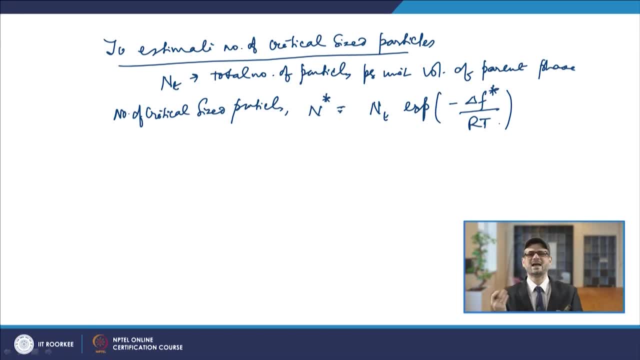 have adjoining atoms on that interface and from that you know parent phase or the liquid phase. one of the atom will jump into that critical sized particle and that will make it supercritical, and then it is said to be nucleated. so if suppose, in that case, if suppose, 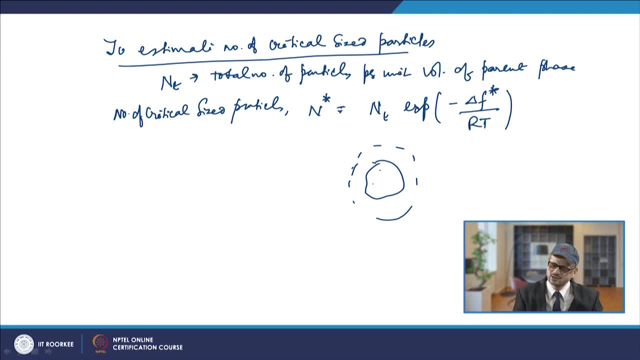 you, this is your product phase and this is your parent phase. so if this is your product phase and this is your parent phase, where you have atoms and this atom has to jump from there to make it, you know, super, you know critical. So if suppose you have S star atoms, which are, you know, which are facing that interface, 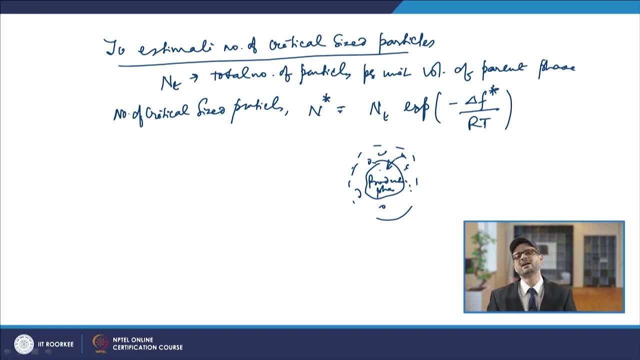 and if one of these S star atoms Divided by RT Is basically jumping into the product phase, then it is said to be nucleated and for that again you are using again these statistical concept and the frequency with which these, any one of these S star atom, that will be crossing that interface. 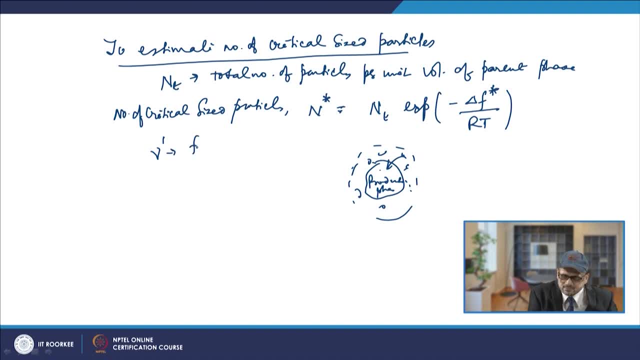 So this nu dash? so if you take nu dash as the frequency with which Any one of S star atoms, S star atoms are the number of atoms which are basically facing this interface or in that parent phase towards the product phase, So if they are, you know they in the atoms can cross the interface, interface and join. 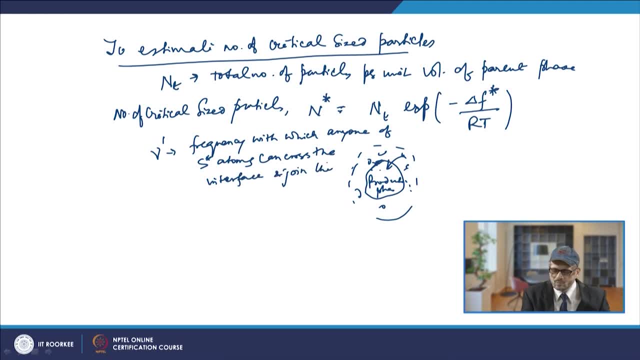 the product phase. Okay, So if that is your nu star, so this nu star also will be taken as S star into nu and exponential of minus delta HD upon RT. So nu is the lattice vibration frequency. so nu is lattice vibration frequency and S star. 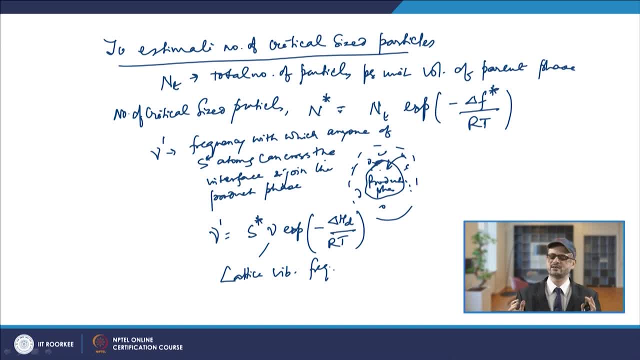 is the number of atoms which are basically across the interface, which are touching, you know, on that surface, And delta HD is the enthalpy of activation. So delta HD will be enthalpy of activation for diffusion across the interface. So if you look at this nu prime value now, that will be S star, nu exponential minus S. 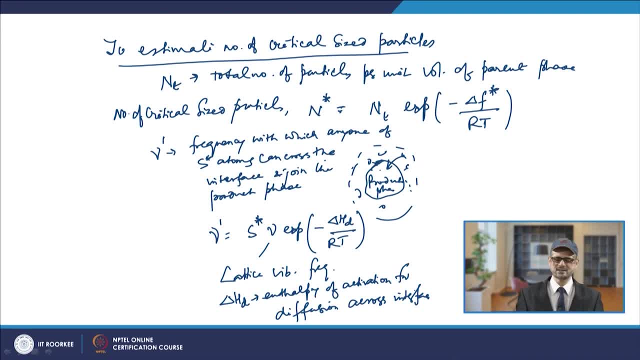 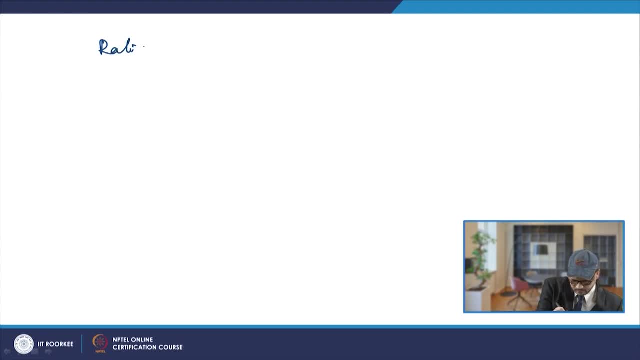 delta HD by RT. Now the thing is that if you talk about the rate of nucleation, So the rate of nucleation of the new phase particle, rate of nucleation of new phase particle, So if you talk about it, it will be, you know. so that will be dn by dt. 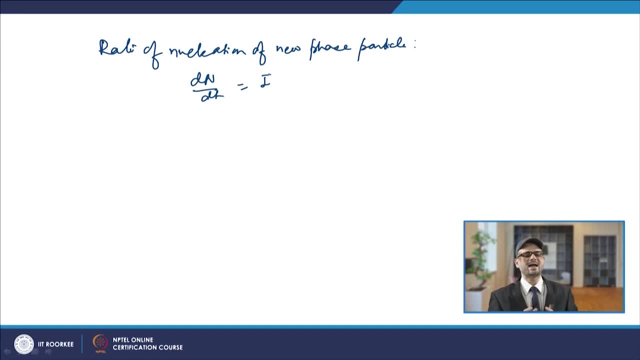 And this we also call it as the I, And it is nothing but the product of the number of critical size particles. so it will be number of critical size particles and multiplied by the frequency with which they try to become super critical. Okay, Okay. 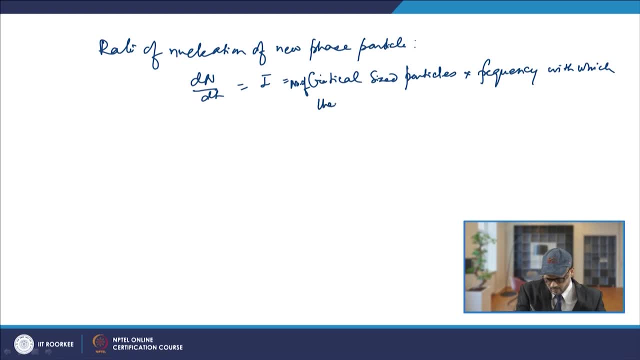 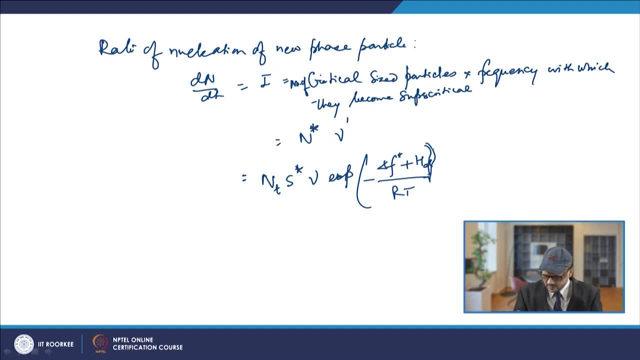 So that basically is talking about- you know the expression- the rate of nucleation and what we see that in this, basically, this pre-exponential term value, it is coming in the range of 10 raise to the power: 42 meter raise to the power minus 3 per. 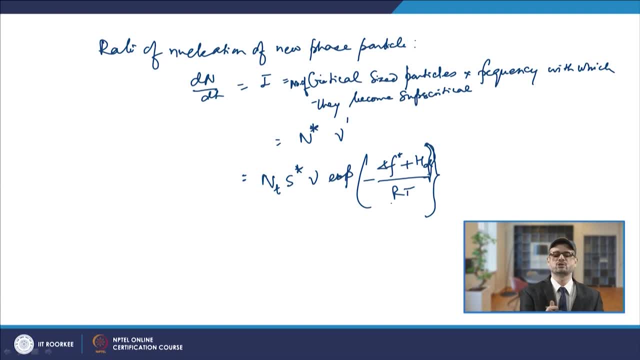 second and then, depending upon these values, your nucleation rate will be defined. So, basically, if you talk about the conditions, like if you are talking about the equilibrium melting temperature, In that case you know, at that point you will have this value as so. depending upon that, 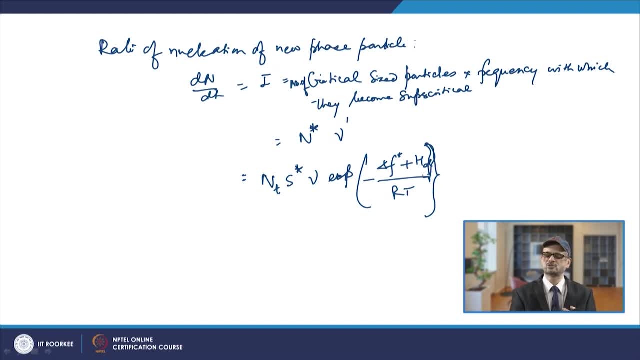 delta, F, star or H d, so depending upon these values at different temperatures. So what is seen? that when you are at a temperature near the equilibrium temperature, at that point also, if you see the rate of nucleation, this rate of nucleation is basically 0.. 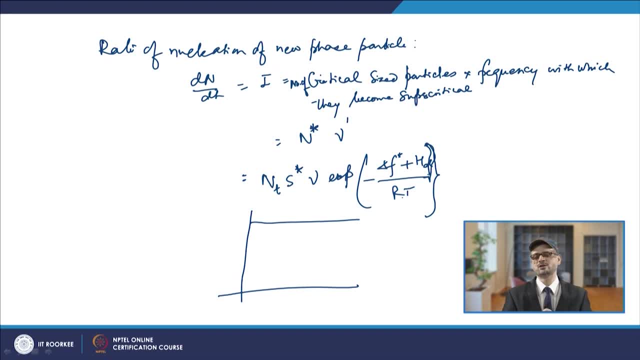 0.. 0. 0. And if you go to the absolute 0 value here, in that case also, it will be- this value will come out to be 0. So what is seen is that if it is temperature and if it is 0 Kelvin and if it is your equilibrium, 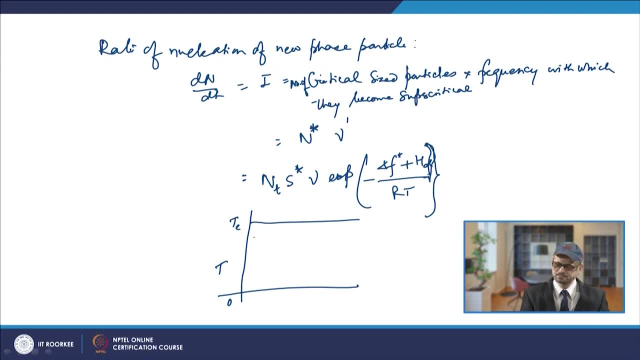 temperature, then what is seen is that your nucleation will proceed from here and then after certain time, basically when this RT term starts dominating. in that case, then it starts decreasing further, So and then it will come to 0 at the 0 temperature. So this is how the rate of nucleation will be. you know, curve will be shown. 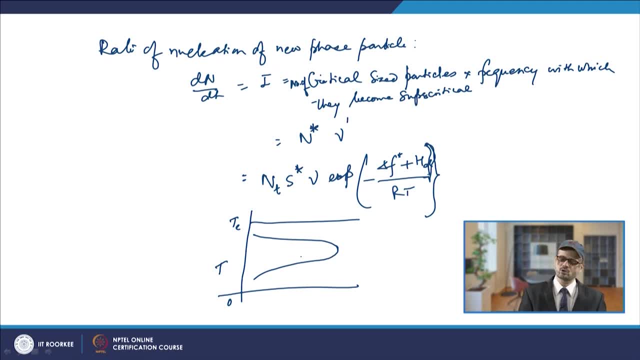 Similar will be the curve for the growth and for growth. basically it will be similar, but it starts, You know, this becomes predominant when you have, you know, the temperature in the upper zone. So your growth also has a similar curve, but it will be more when it is near to the equilibrium. 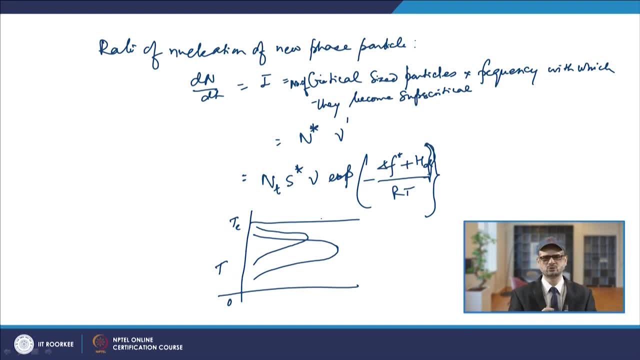 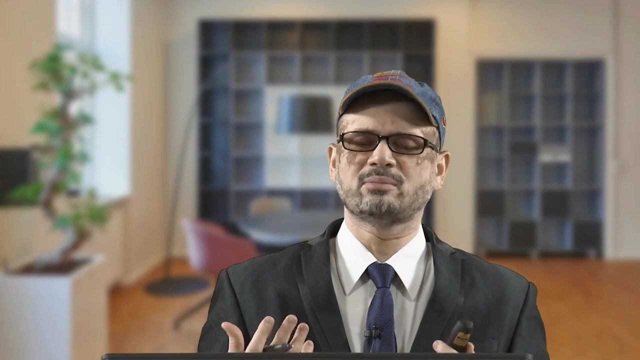 temperature and depending upon these two, you will have the transformation curve. So you will have the transformation curve, dx by dt, which will be in between. So this is the concept of transformation in between in the case of you know the materials Now. so this was the concept of transformation in the case of homogeneous nucleation. 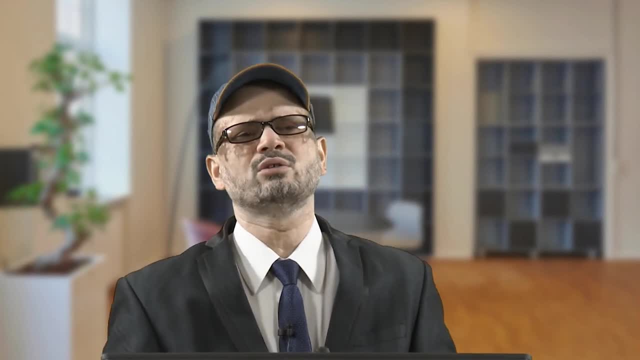 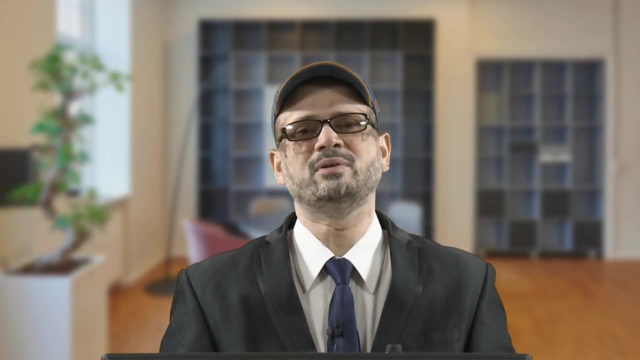 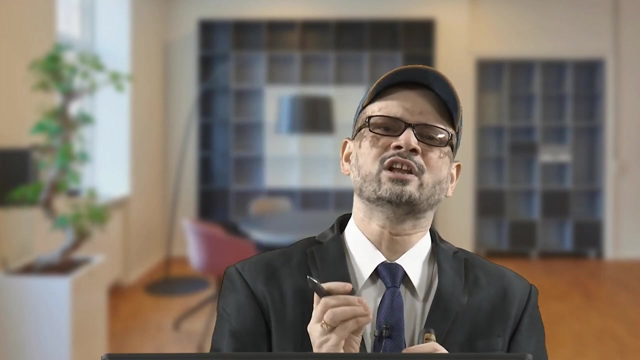 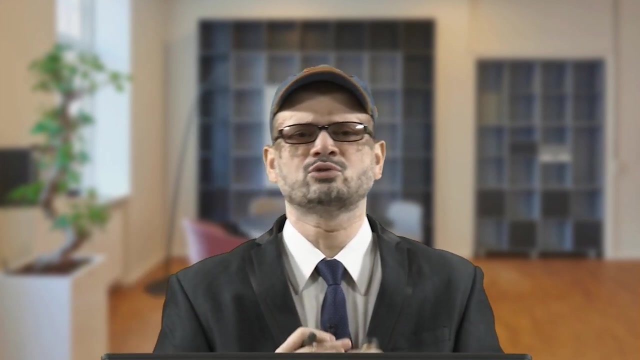 When we talk about the heterogeneous nucleation now, heterogeneous nucleation at preferred places you will have, the chances of nucleation will be more. That is basically governed based on the, you know, the particle which is nucleated and the interface which is created. So taking upon the surface tension, you know, forces also into account and other factors. 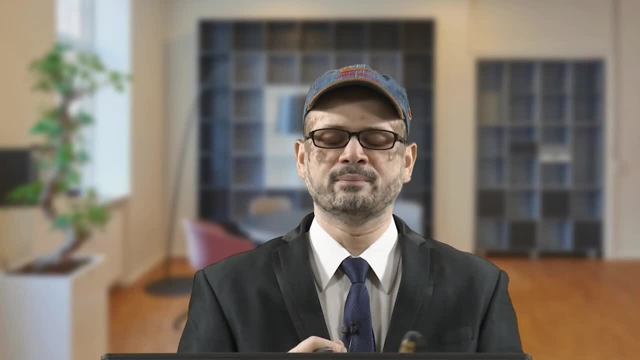 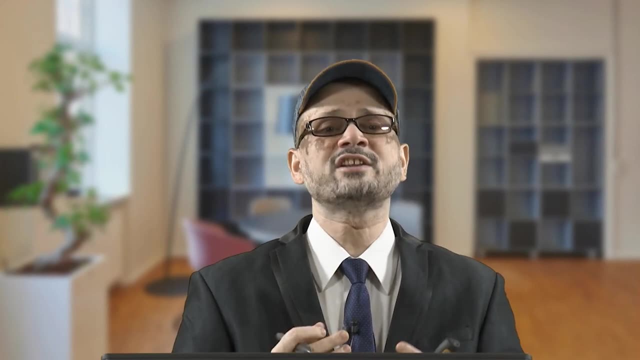 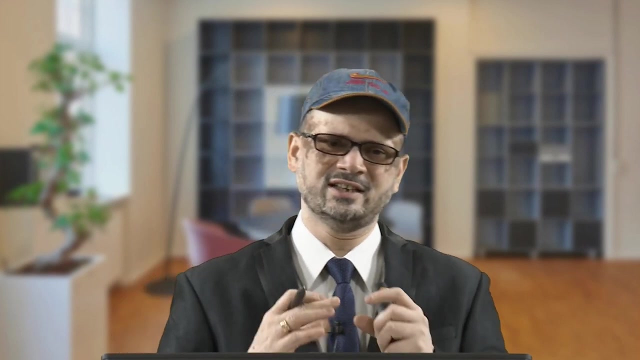 so, summation of forces, if you do, if you read them from some standard books. So the thing is that the energy which you have to supply for creating the surface in the case of homogeneous nucleation, That basically, is less in the case of heterogeneous nucleation, because here you have certain 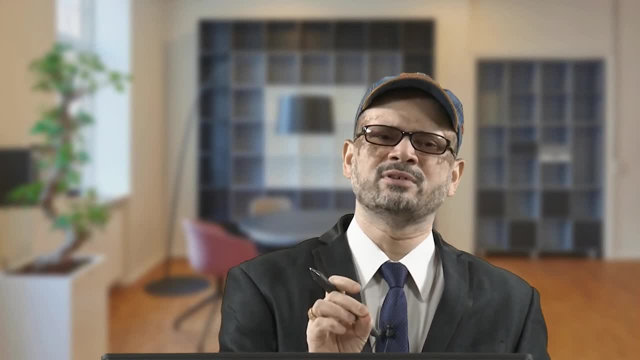 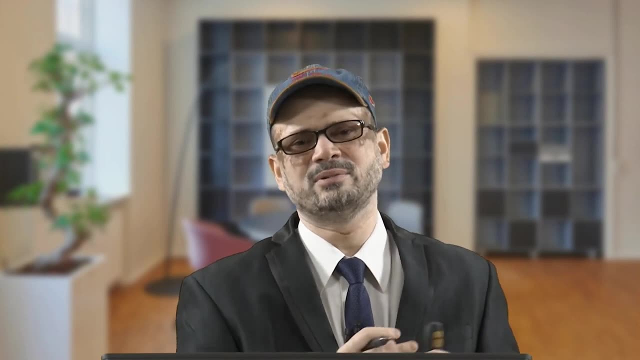 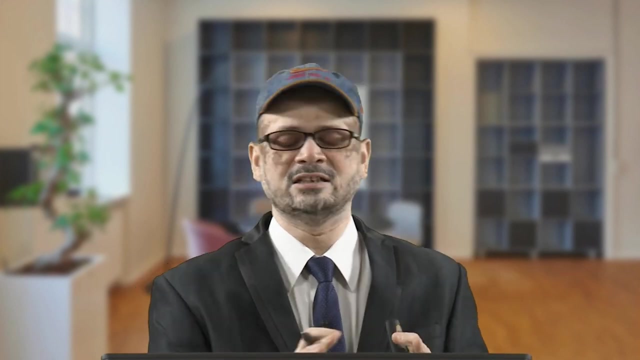 surfaces present. Now that may be in the form of inclusions, or that may be the wall of the container, which is basically the sand, basically sand molding material. you have inclusions. So basically, in that case that becomes your source and from there the nucleation is basically. 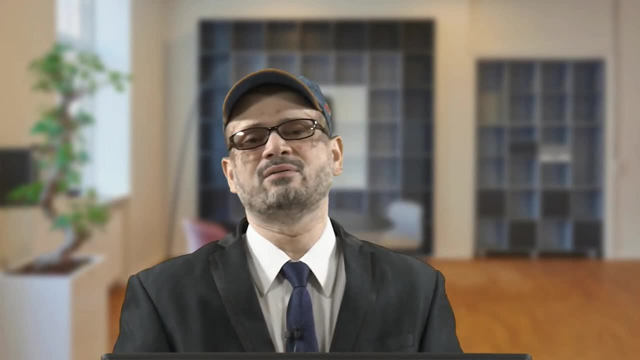 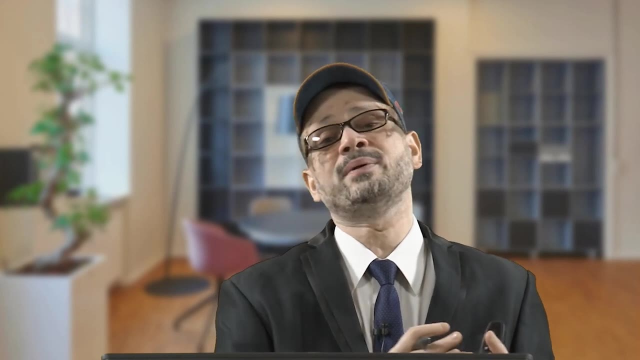 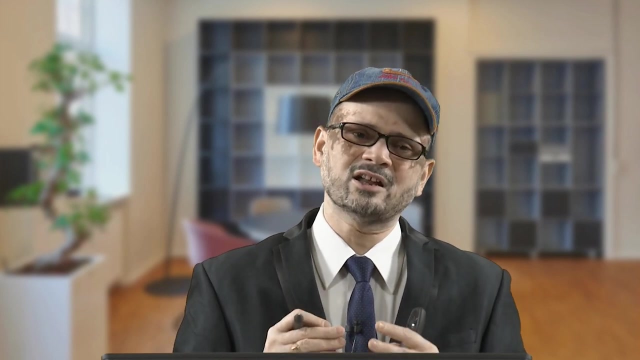 assisted. So the delta F star value which you are getting in the case of homogeneous nucleation: In the case of heterogeneous nucleation it may be so maximum it will be the same as homogeneous nucleation. for certain cases, However, depending upon the characteristics of the product particle and the interface, 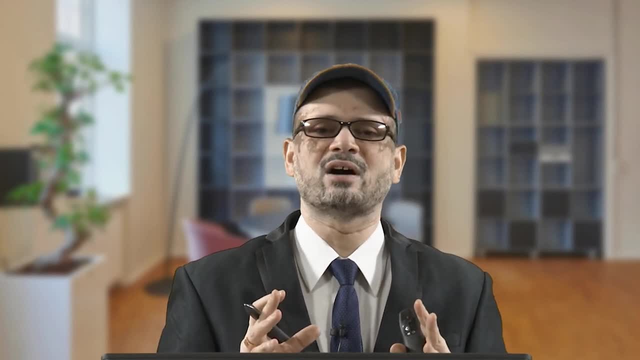 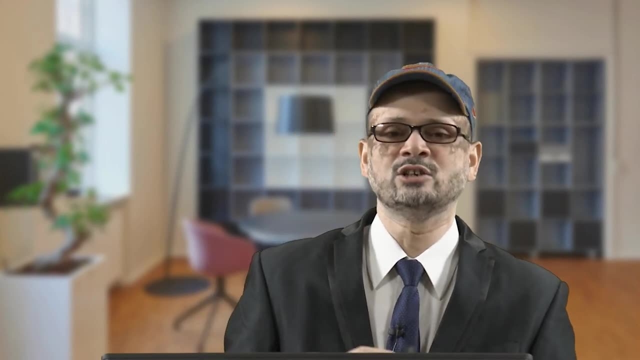 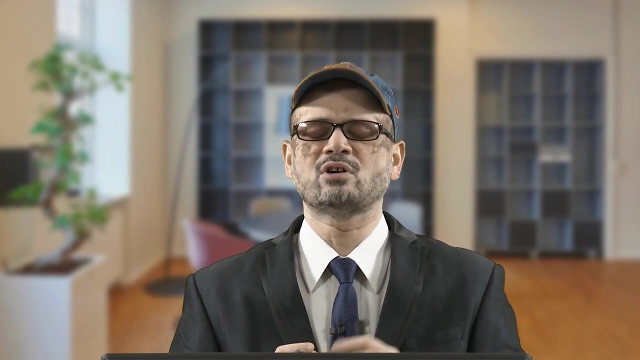 or so you will have. the delta F star requirement will be lesser and that will basically giving you know The ease in nucleation and that is why that is the concept of heterogeneous nucleation. So so we will be, whenever we will be talking about the transformation of the you know from, 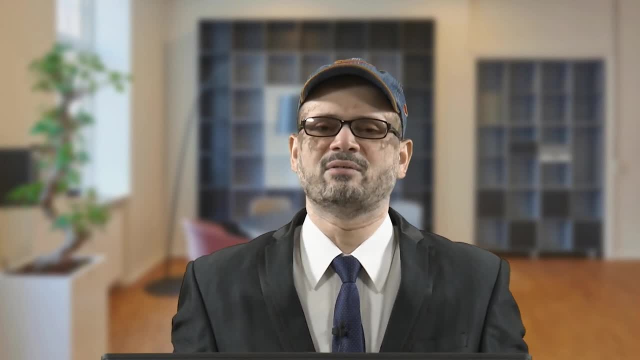 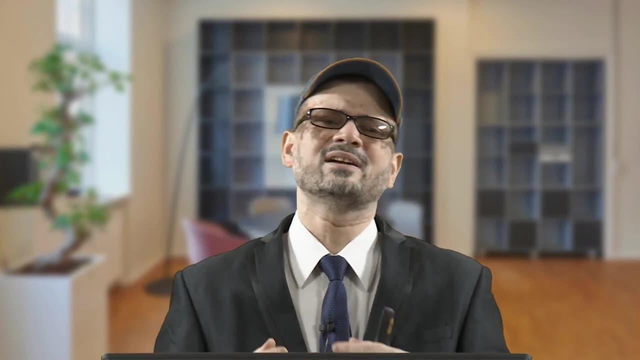 one phase to other. all these things must be our in our mind So that we can correlate that what might have happened. This is from the liquid to solid state. similar thing happen in the case of solid to solid state transformation. Now, in those cases you have other strain, energy factor. 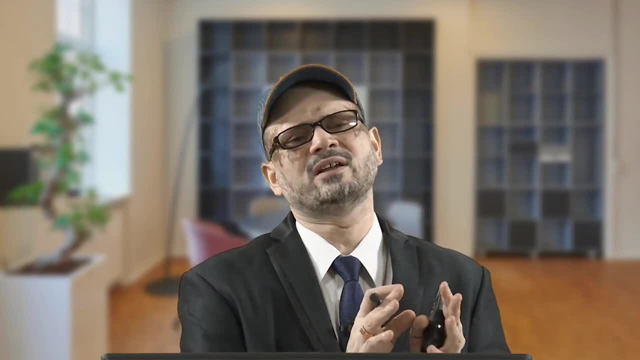 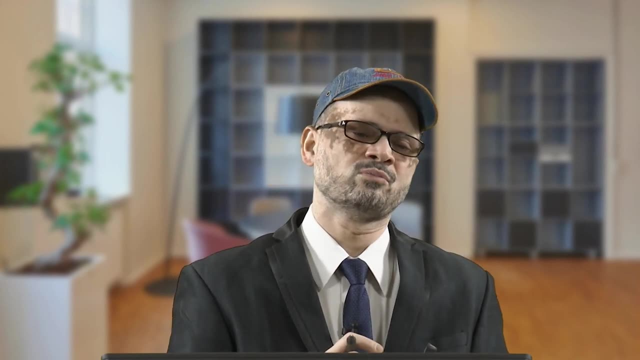 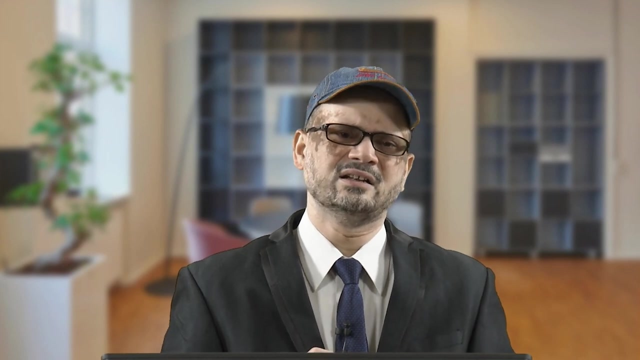 So this strain factor is coming into picture. So basically, there also you will have nucleation and you may have nucleation at certain points. Many a times what we see, that you have certain preferred places where the nucleation starts and that will be at those higher energy places, like you have grain boundaries or the dislocation. 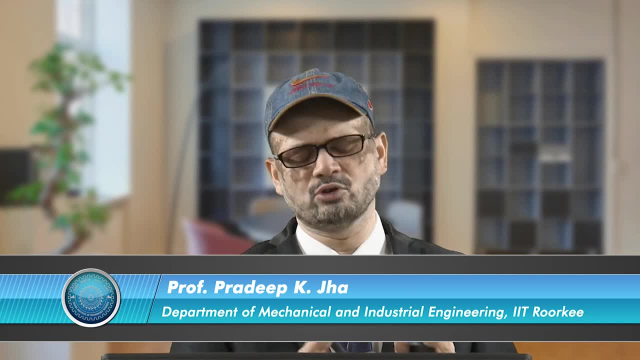 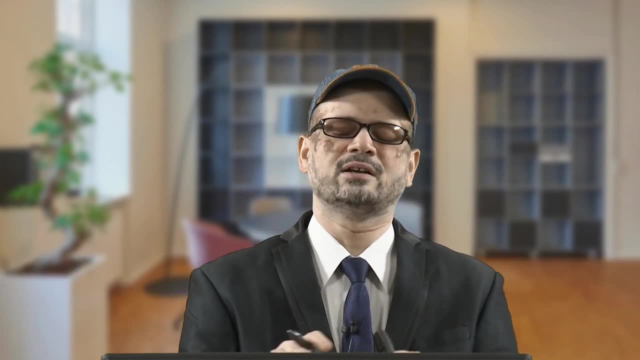 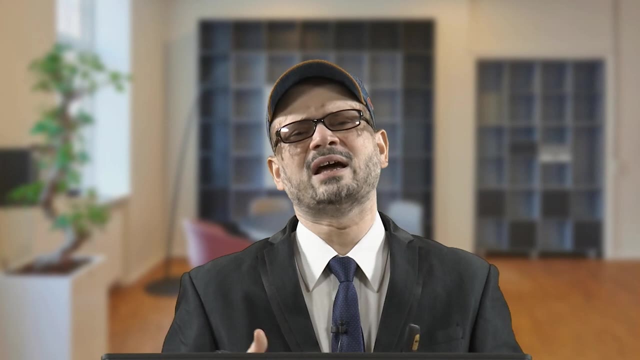 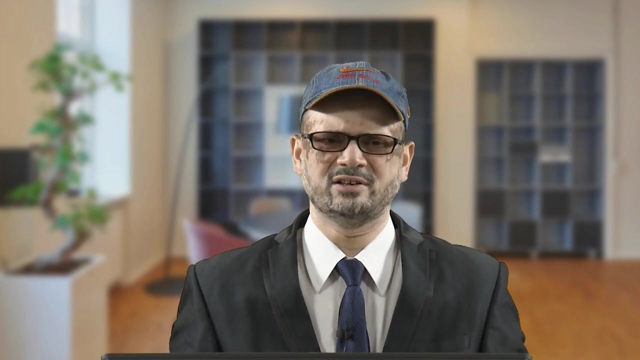 sites or so, So, so, so, that will So basically, So, So what free energy values concept, and also you know other. whatever we have understood, we must have the clarity of these concepts in mind so that it will assist us in the understanding of other- you know metallurgical processes or the welding processes in a better manner.